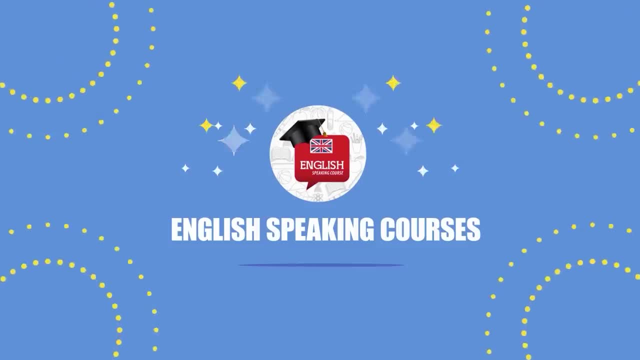 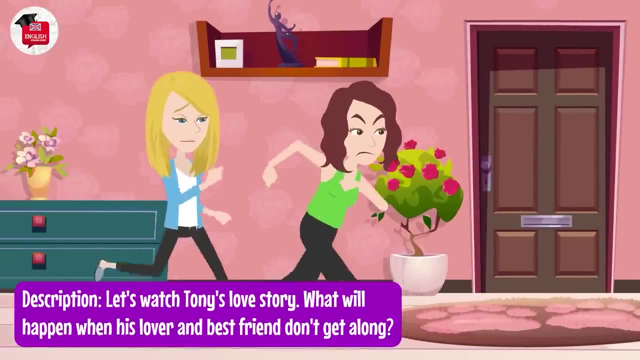 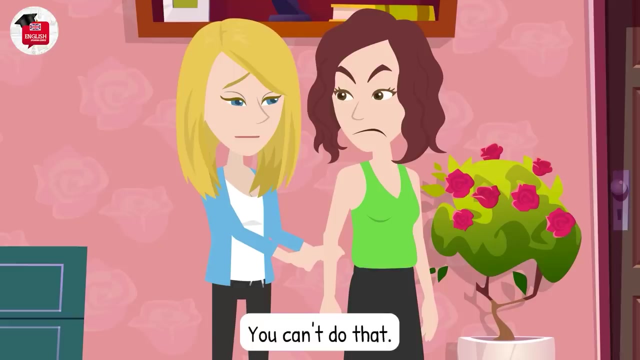 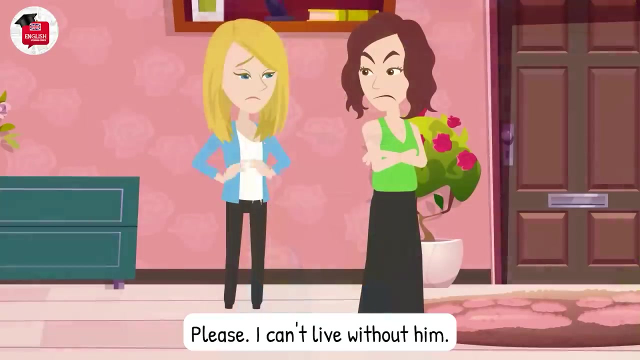 Let's watch Tony's love story. What will happen when his lover and best friend don't get along? Please, don't do it. You can't do that. I love Tony so much. I can't leave him, Please. I can't live without him. 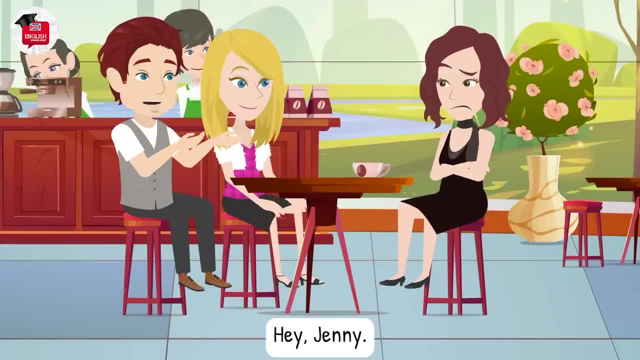 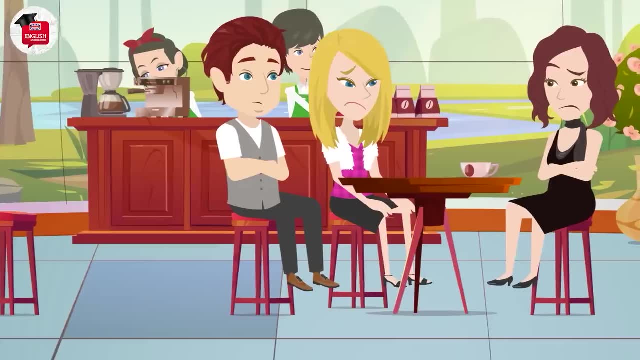 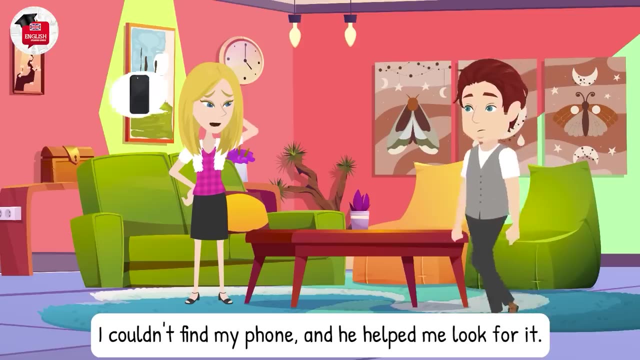 Hey Jenny. Hi Tony, You're 20 minutes late. Sorry, Jenny, I'm the one who needs to be sorry, not Tony. He came to pick me up. I couldn't find my phone and he helped me look for it. 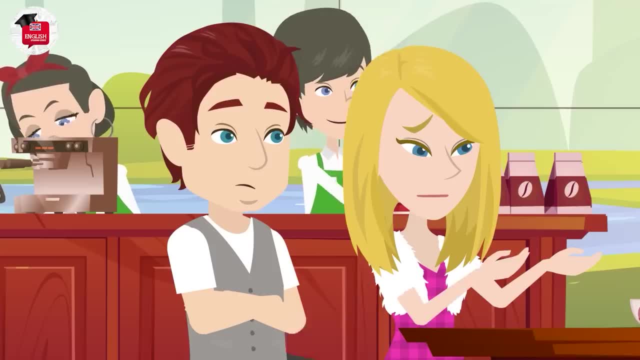 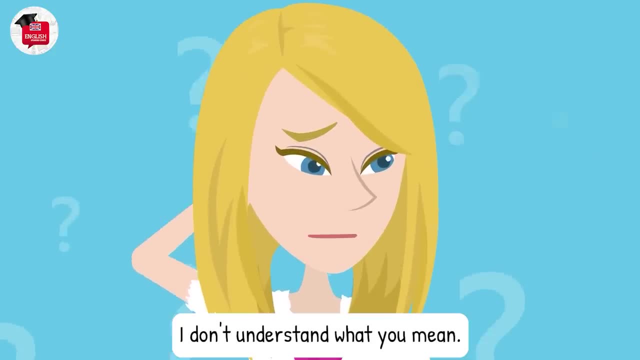 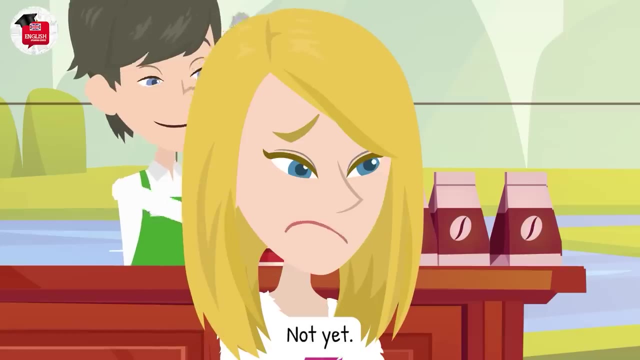 Hmm, okay, Sorry. Did you really lose your phone or did you hide it? I don't understand what you're talking about. I don't understand what you mean. Come on, Jenny. So have you found the phones yet? Not yet. 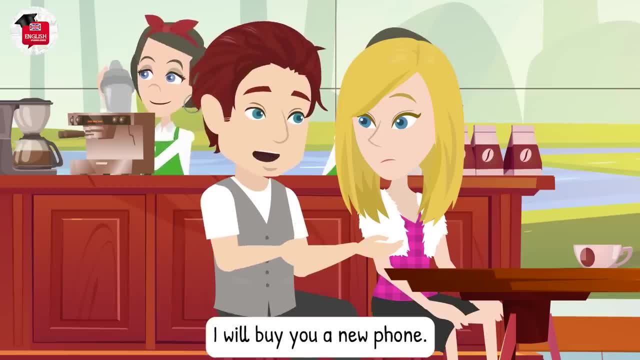 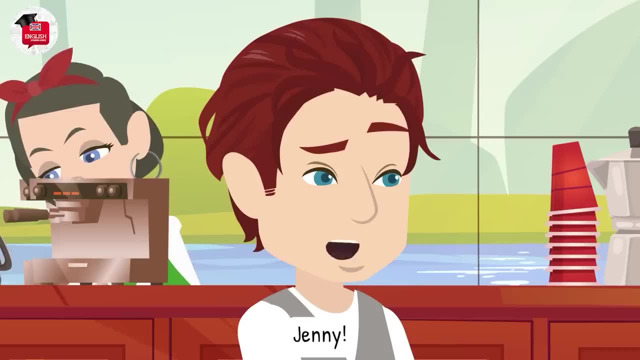 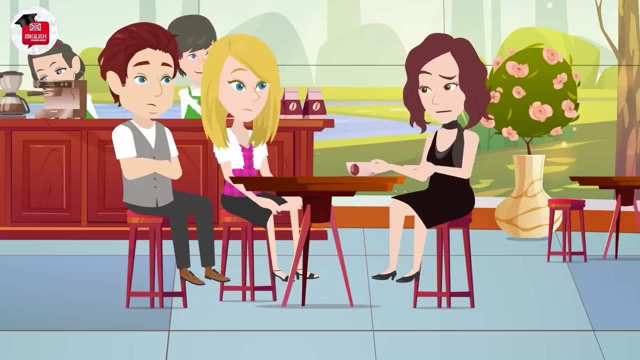 It's okay, Alice, Don't be sad, I will buy you a new phone. You should be careful or you will lose both money and love Jenny. Okay, whatever. So is she your new girlfriend? Yes, she is, Alice. 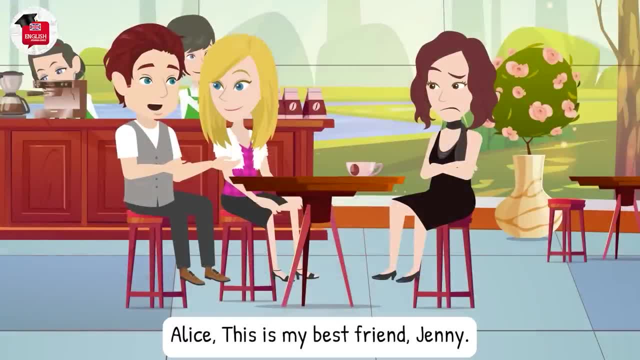 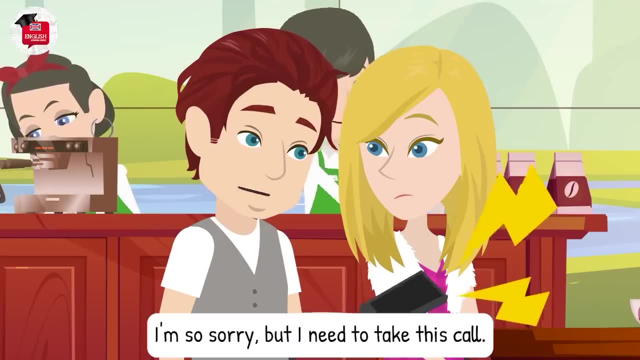 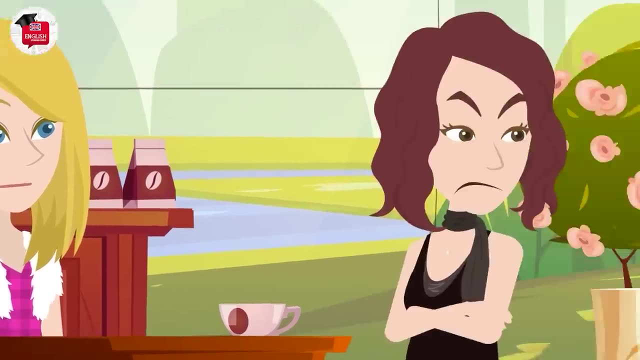 She is my lovely girlfriend Alice. this is my best friend, Jenny. I'm so sorry but I need to take this call. I'll be right back Nice to meet you, Jenny. It's not nice at all to meet you, Alice. 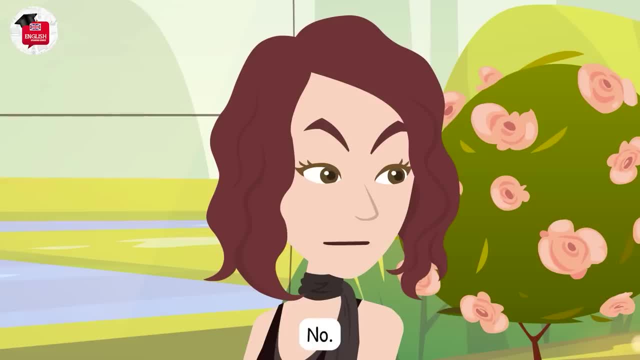 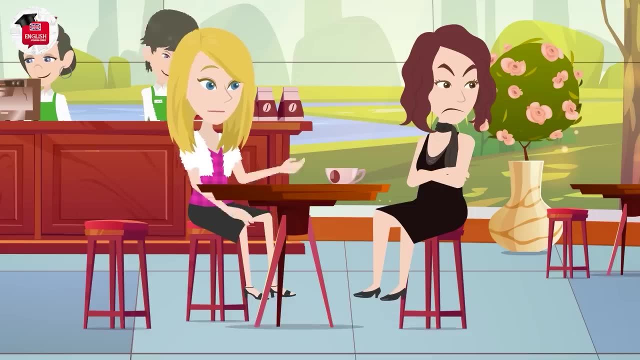 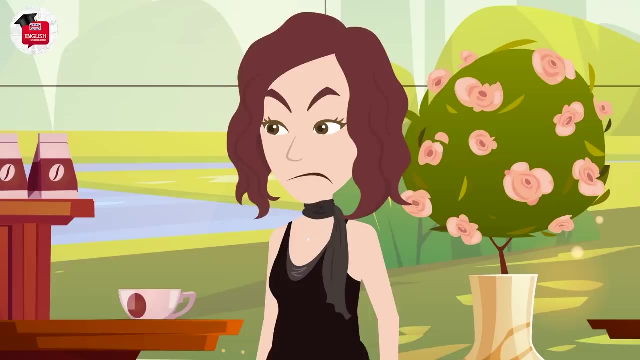 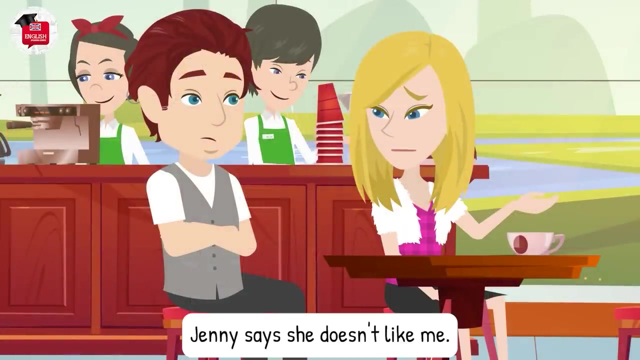 You don't like me, do you? No, Why? We just met. What is it about me That makes you dislike me? Alice, listen, Stay away from Tony. What happened? I have to go now, Talk later. Jenny says she doesn't like me. 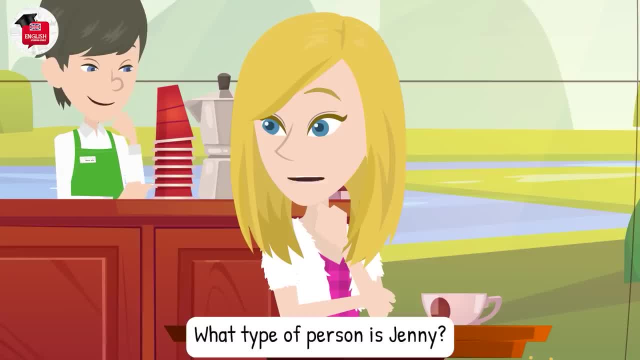 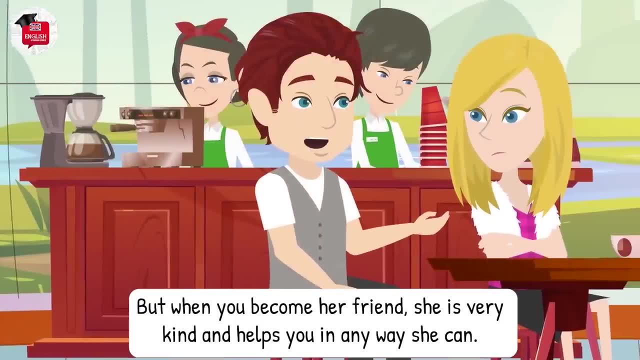 Don't worry, Alice. What type of person is Jenny? She is hot-tempered and hard to please, But when you become her friend, she is very kind and helpful. But when you become her friend, she is very kind and helpful. 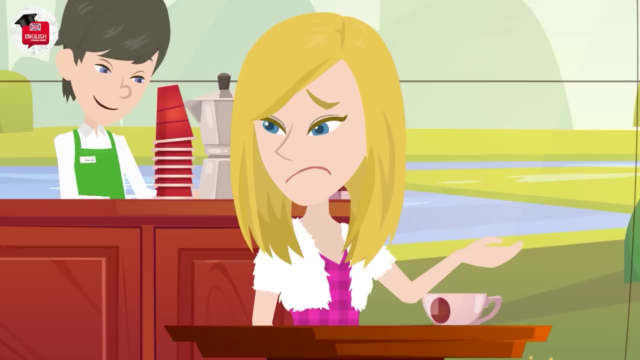 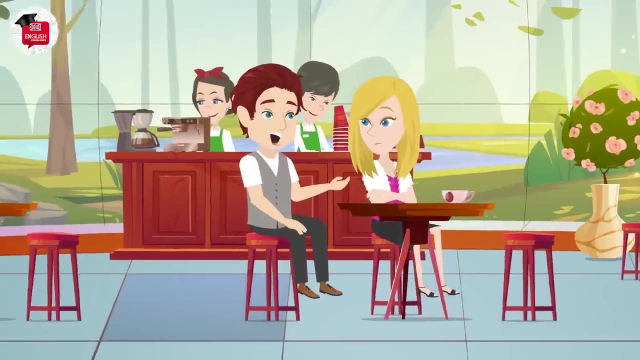 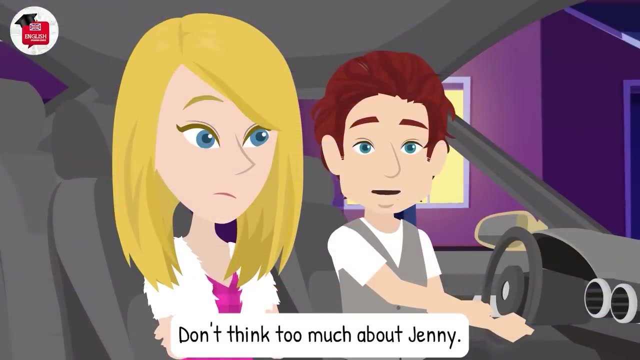 But when you become her friend, she is very kind and helpful. She helps you in any way she can. I hope she will like me more in the future. She will Believe me. Don't think too much about Jenny. Just take a shower, watch your favorite movie and get a good night's sleep. 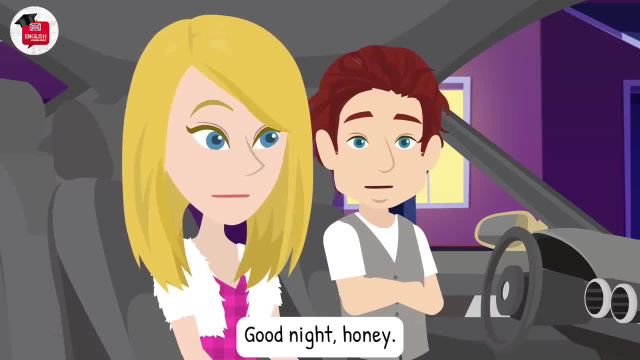 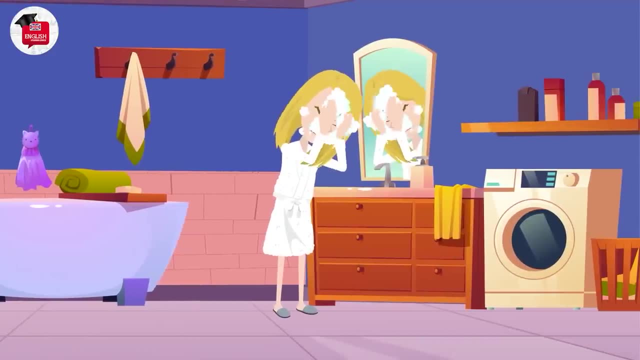 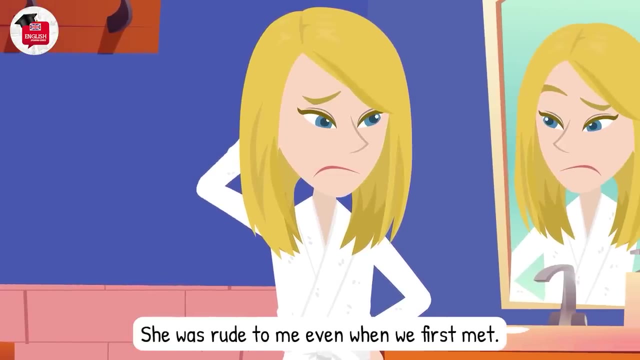 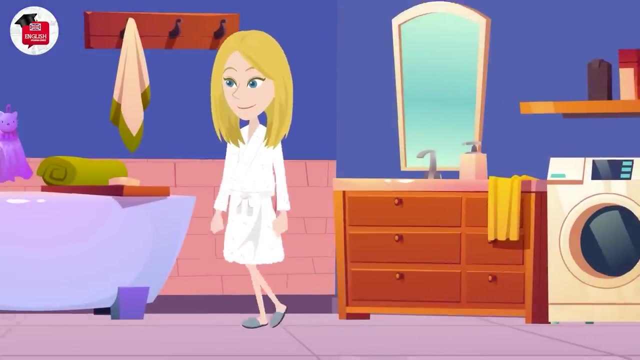 Okay, Tony, Good night. Good night, honey. Good night. There's something about Jenny that I don't know. She was rude to me even when we first met. Maybe I can find out more about her on social media. Oh, why doesn't she update her status? 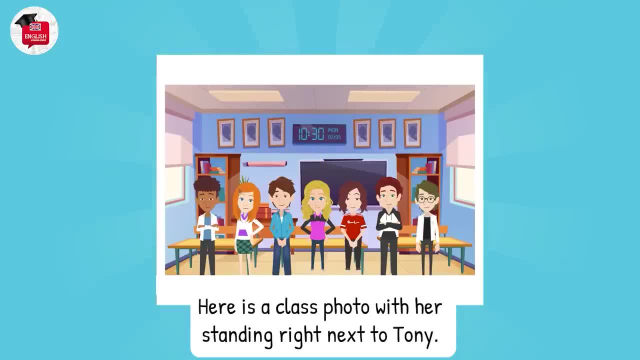 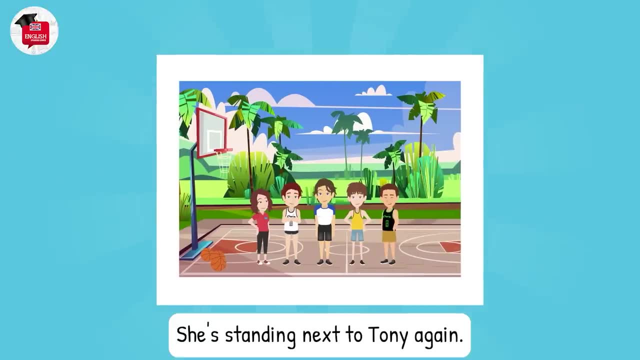 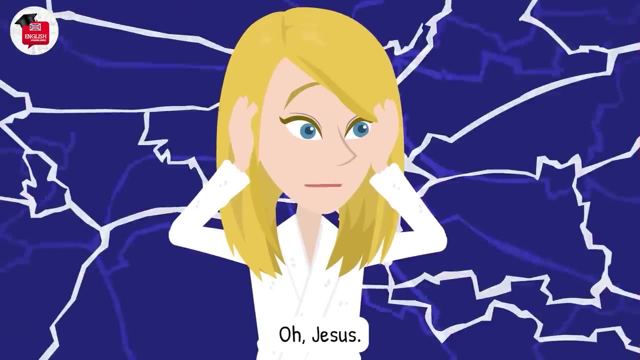 Oh, Here is a class photo with her standing right next to Tony, standing right next to tony. picture of her and the basketball team. she's standing next to tony again. look at the way she looks at tony. oh jesus, maybe she likes tony. that's why she treated me. 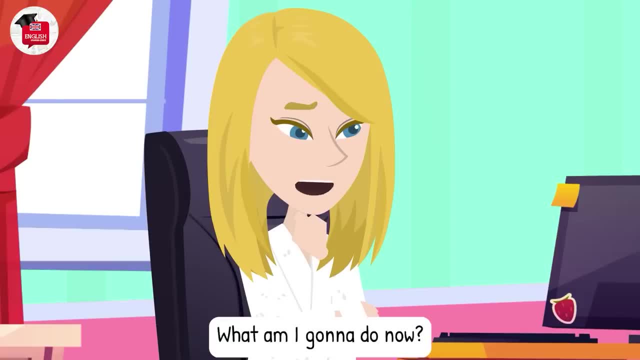 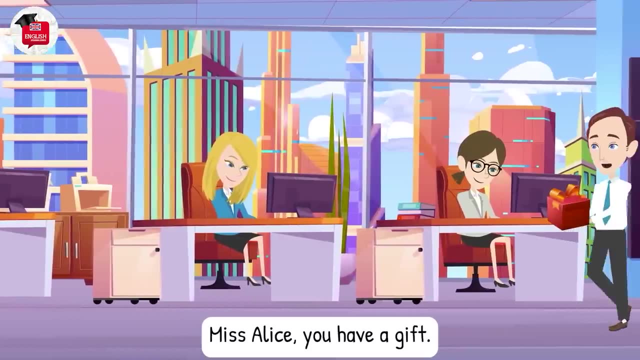 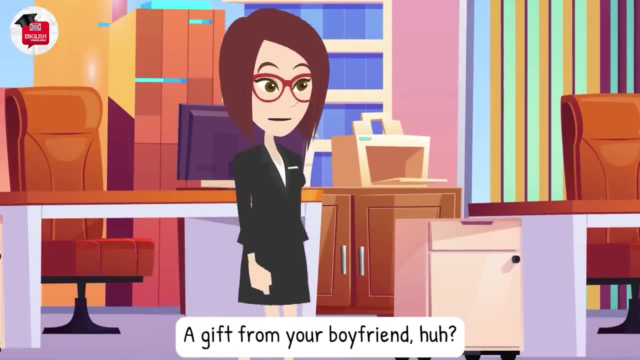 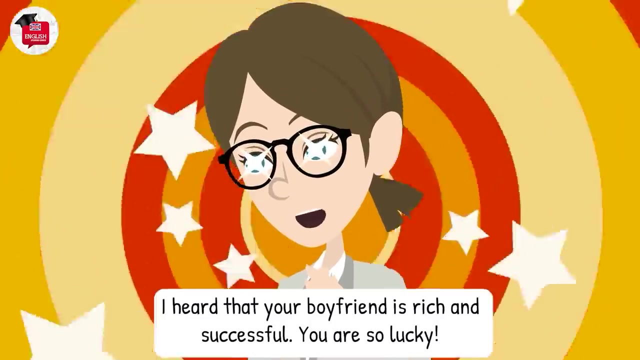 rudely. what am i gonna do now? miss alice, you have a gift here you are, thank you, a gift from your boyfriend. huh, i don't know. i heard that your boyfriend is rich and successful. you are so lucky. open it, alice. i'm curious to see open. 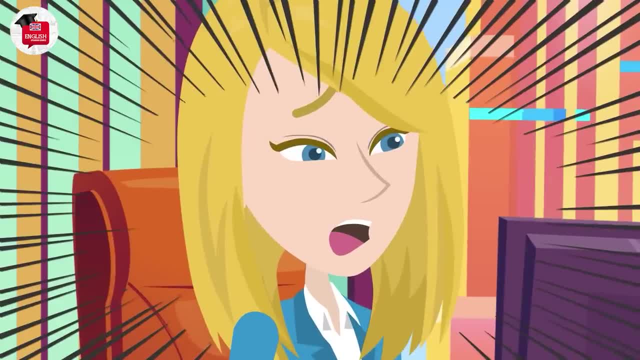 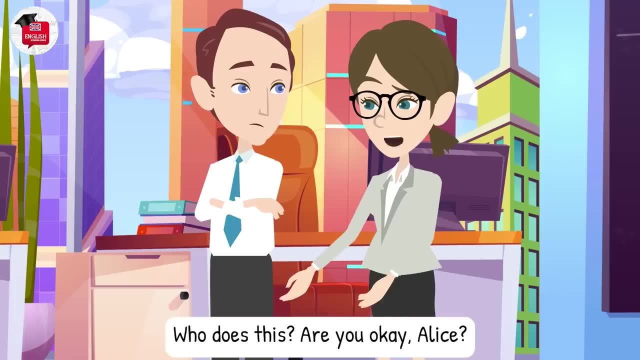 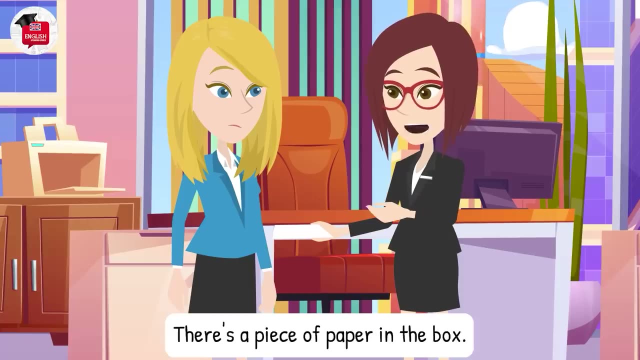 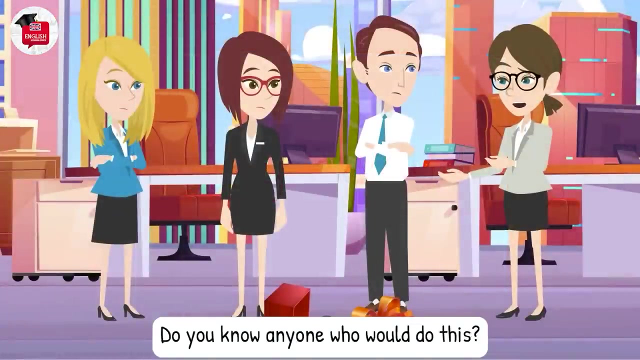 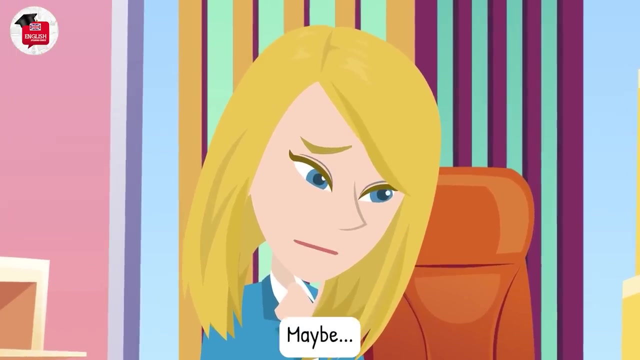 are they snakes? yeah, but they're fake. who does this? are you okay, alice? i'm fine. thanks, bella. uh, there's a piece of paper in the box, stay away. do you know anyone who would do this? that's so rude and creepy. hmm, maybe. what are you saying? do you know who did this? 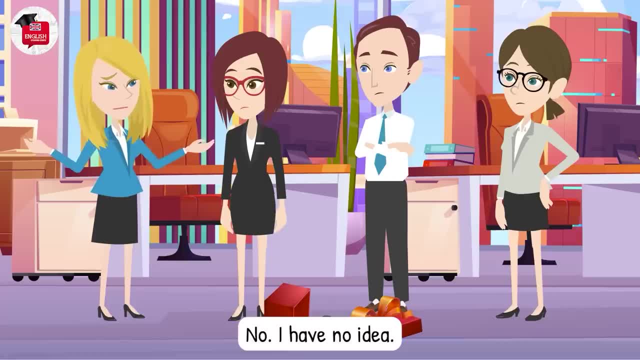 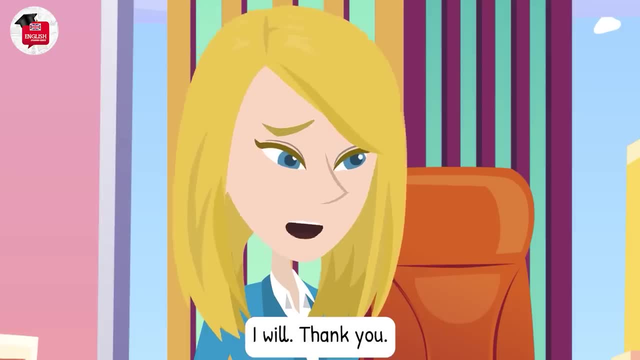 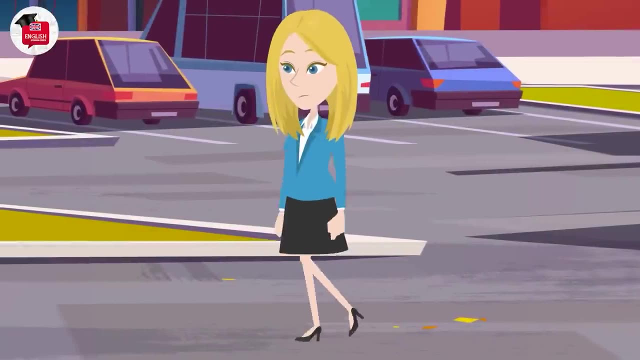 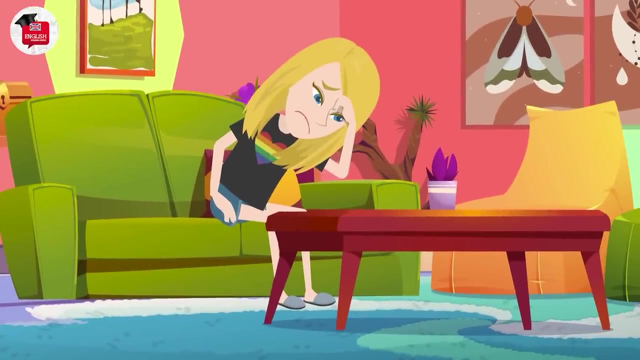 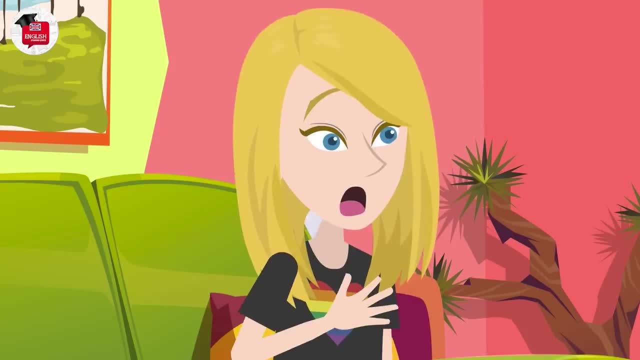 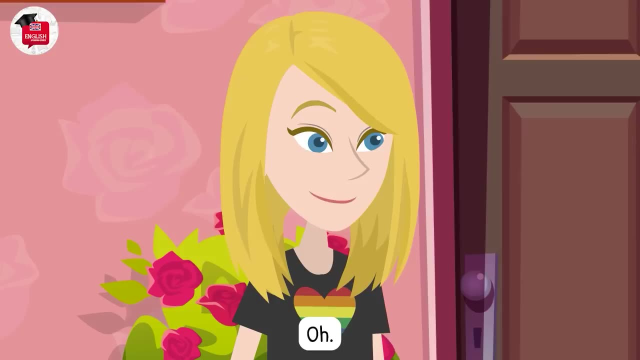 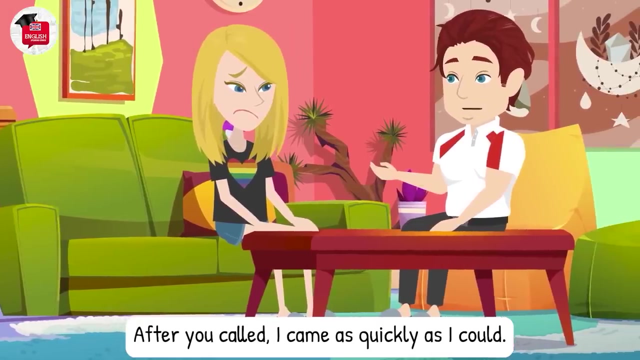 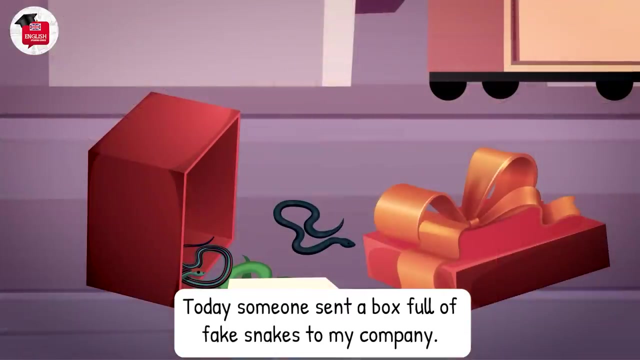 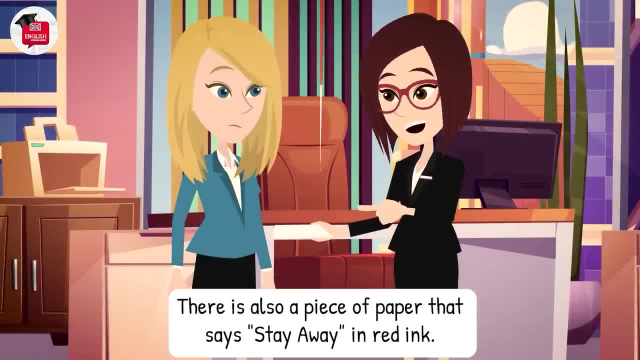 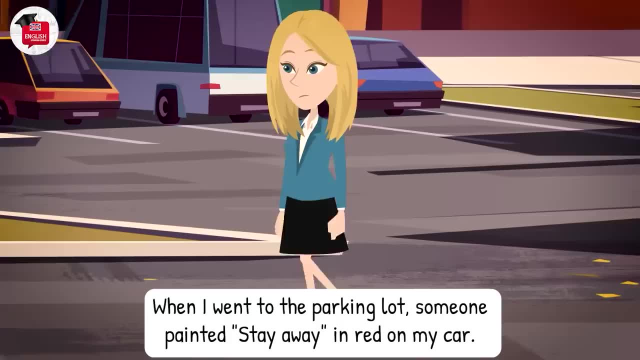 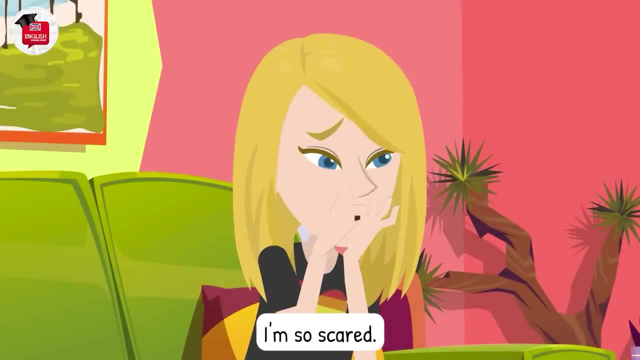 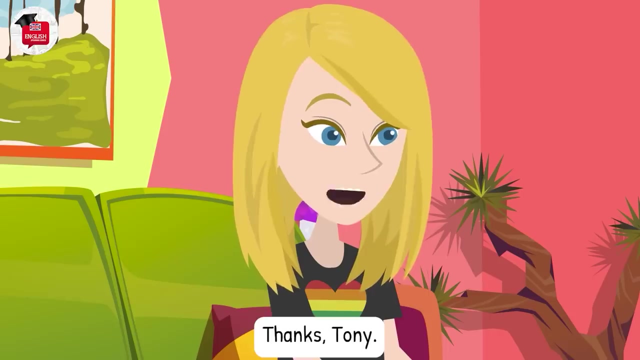 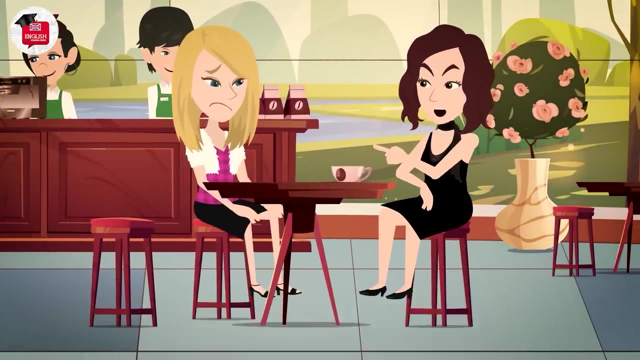 there's also a piece of paper that says stay away, in red ink. oh my god, who did that? when i went to the parking lot, someone painted stay away and read on my car. i'm so scared. i'm here now. i'll drop you off at work and pick you up. thanks, tony. the last time i met jenny, she also told me to stay away from you. do you think she did this? 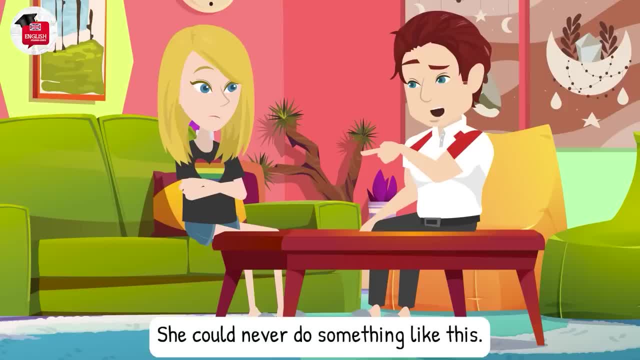 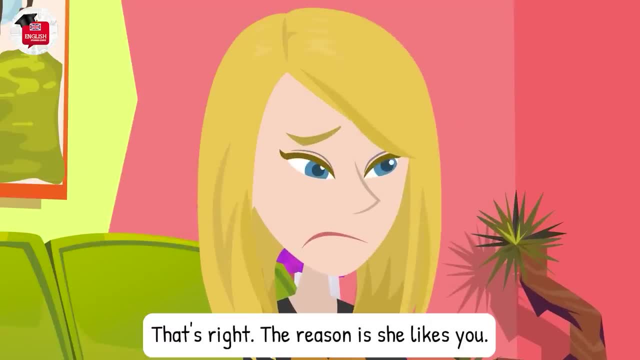 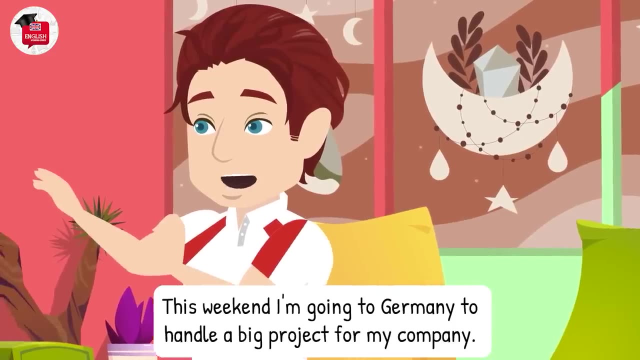 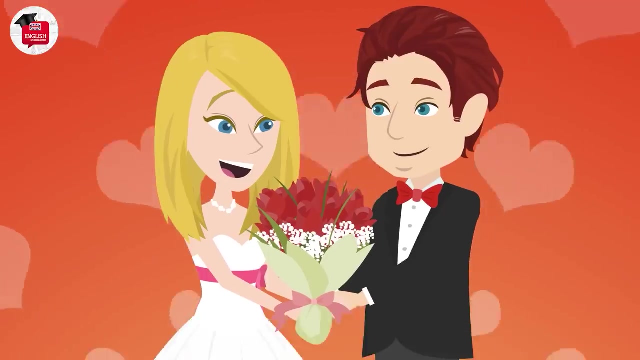 no, alice, she could never do something like this. she does everything for a reason. that's right. the reason is she likes you. don't worry, alice, nothing will happen to you. this weekend i'm going to germany to handle a big project for my company. when i return, i will prepare for our wedding. 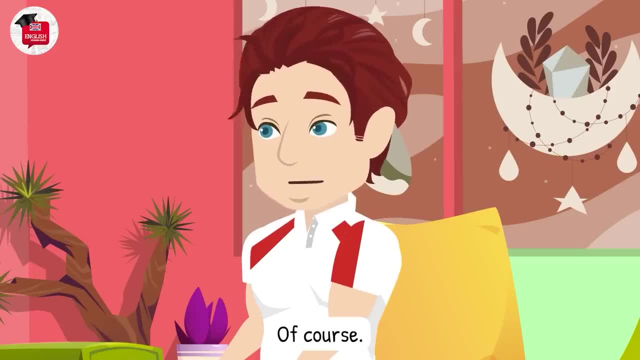 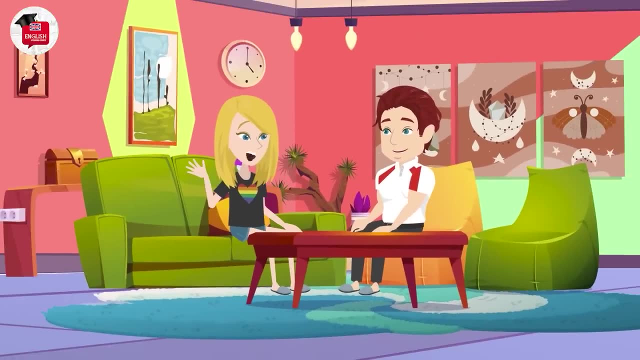 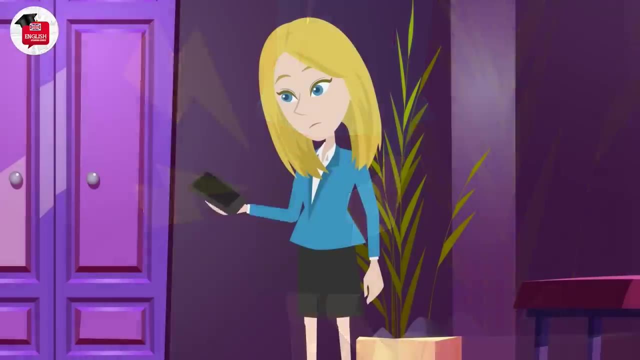 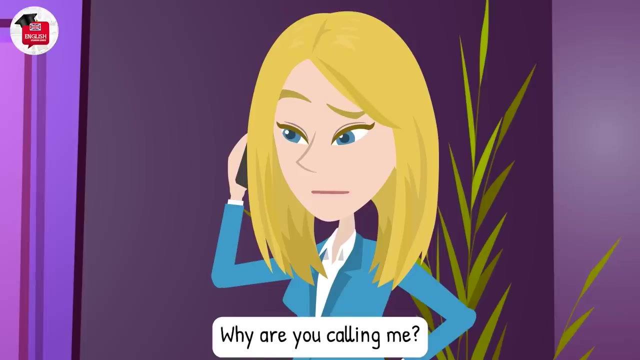 really, of course. oh, tony, i can't wait. hello, it's jenny, tony's best friend. hi, jenny, why are you calling me? let's meet. i have something to tell you. we can talk on the phone. no, i want to see you. why, jenny? 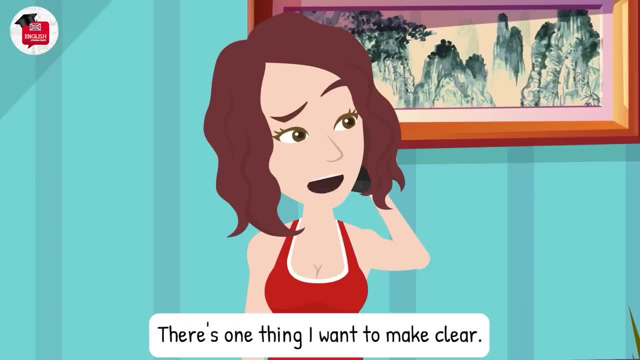 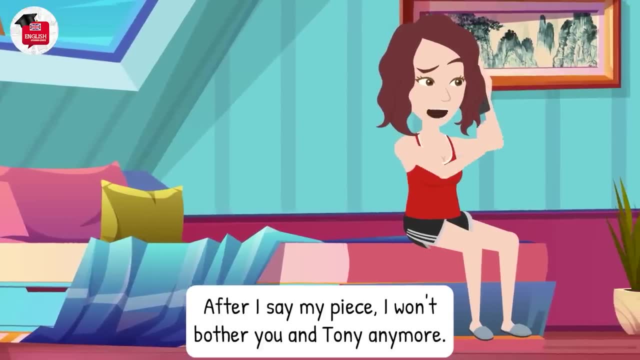 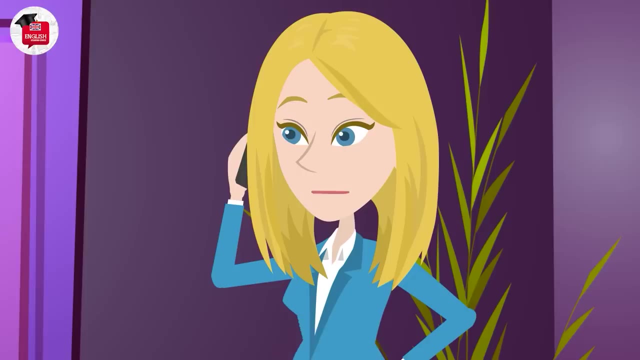 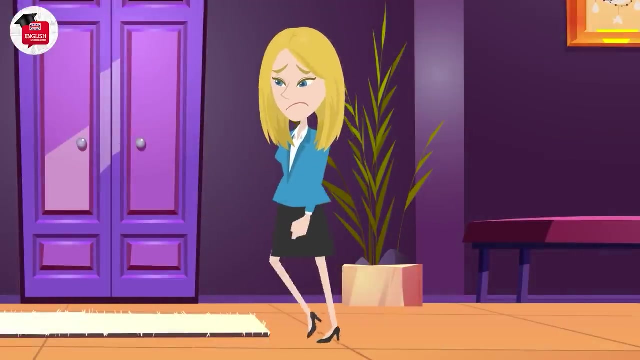 there's one thing i want to make clear. i have nothing to say to you after i say my piece. i won't bother you and tony anymore, i promise. okay, jenny, the condition is that we meet at my house, okay, well, what are we going to eat when we get home then? 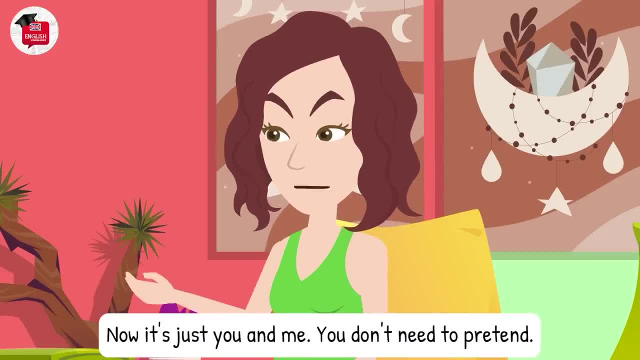 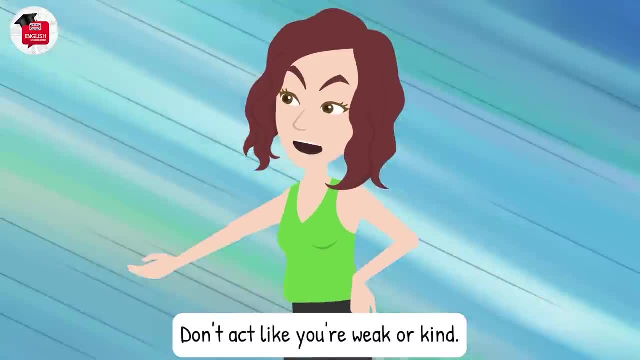 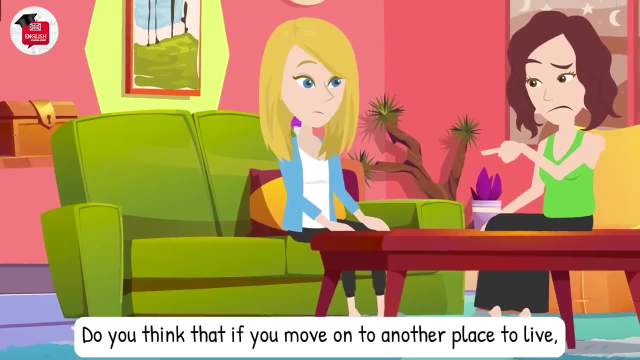 to say: alice, now that it's just you and me, you don't need to pretend. what do you mean? don't act like you're weak or kind. that's not who you are. please stop it, jenny. do you think that if you move on to another place to live, people will keep forgetting what you did in the past? 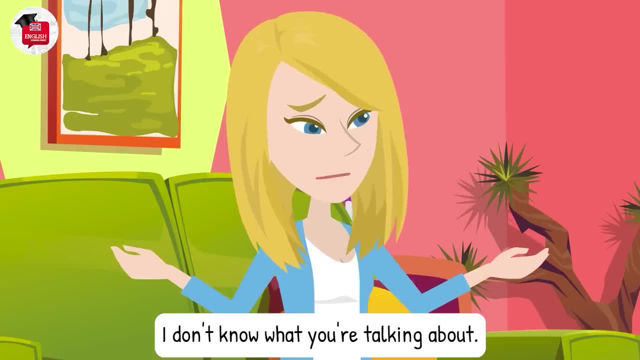 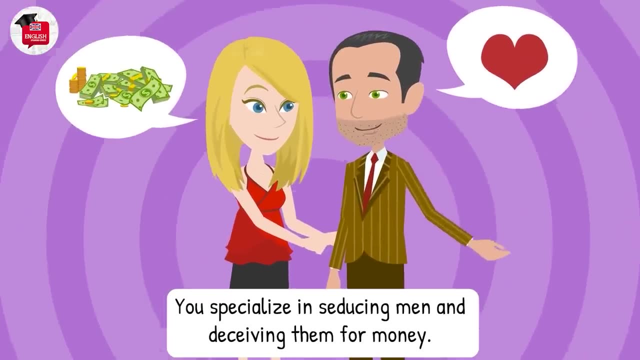 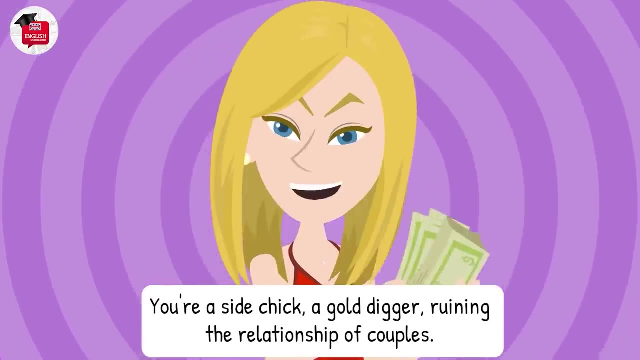 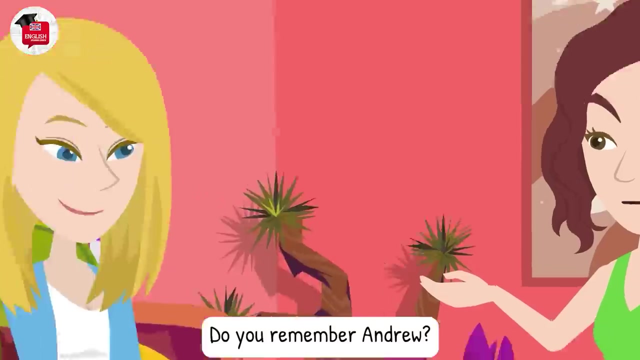 i don't know what you're talking about. i know you well, alice. you specialize in seducing men and deceiving them for money. you're a side chick, a gold digger, ruining the relationship of couples. you should be careful with your words. do you remember andrew andrew, i'm his ex-girlfriend. 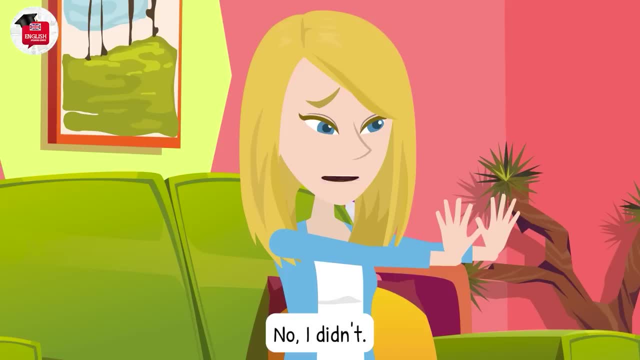 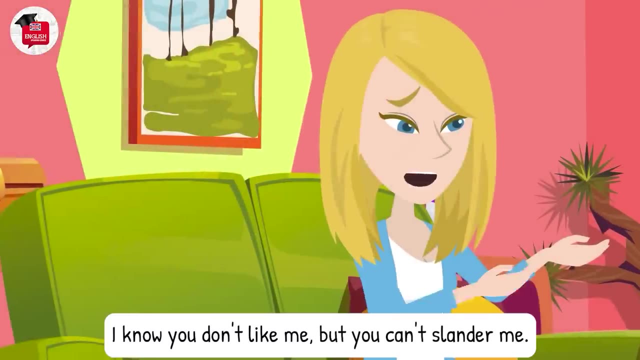 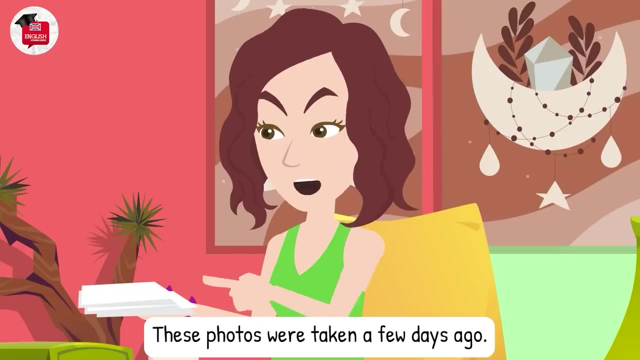 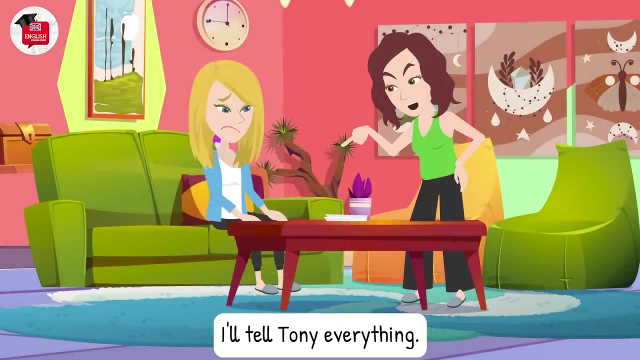 and you took him away from me. no, i didn't. maybe you don't recognize me, but i will never forget you. i know you don't like me, but you can't slander me. these photos were taken a few days ago. you're dating someone else, while you're getting married to tony. i'll tell tony everything. 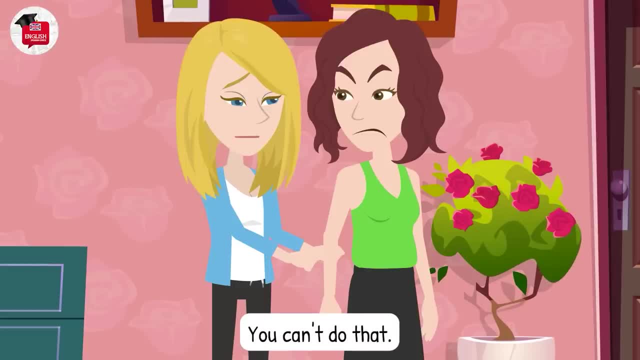 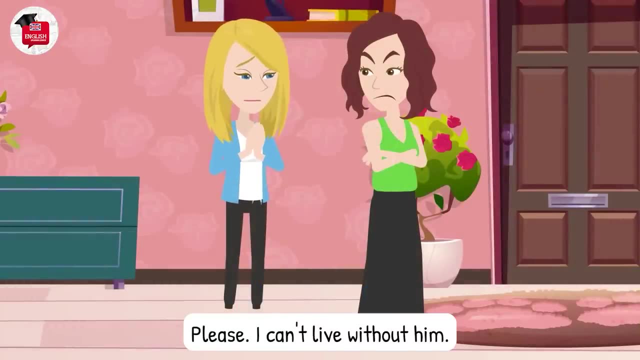 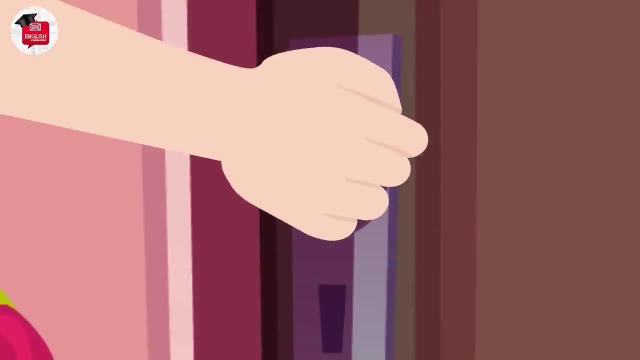 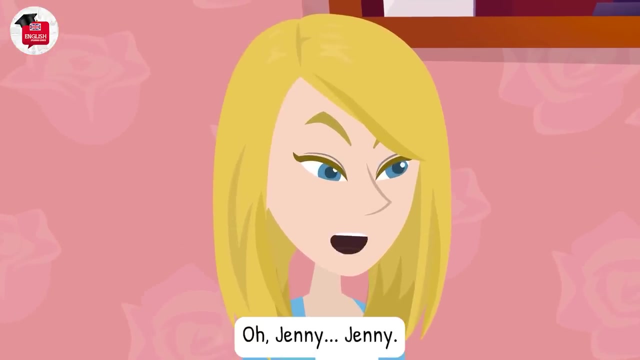 please don't do it. you can't do that. i love tony so much. i can't leave him please. i can't live without him. you don't love him, you just want his money. why is this door locked? let me go. oh, jenny. jenny- actually the first time i met you at the restaurant. 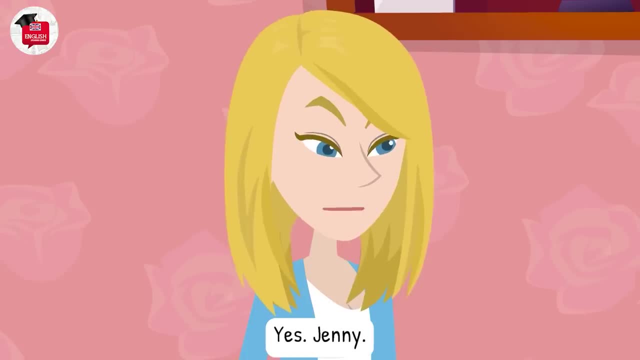 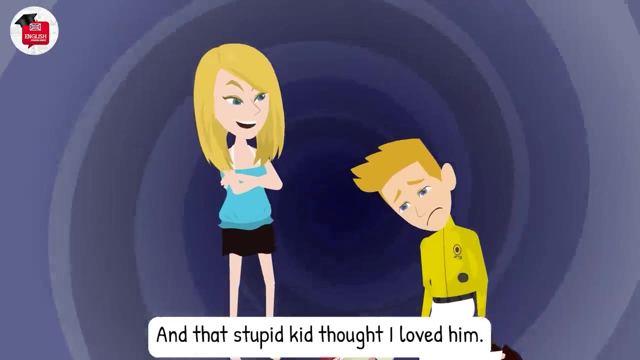 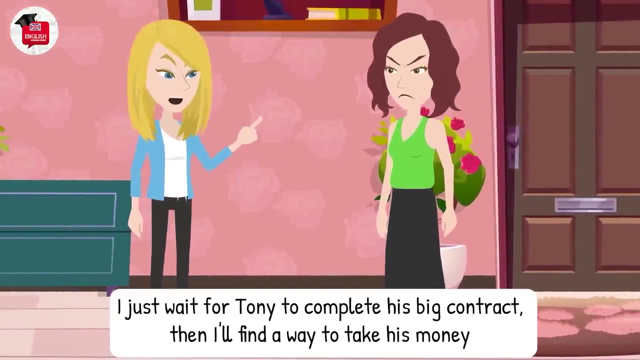 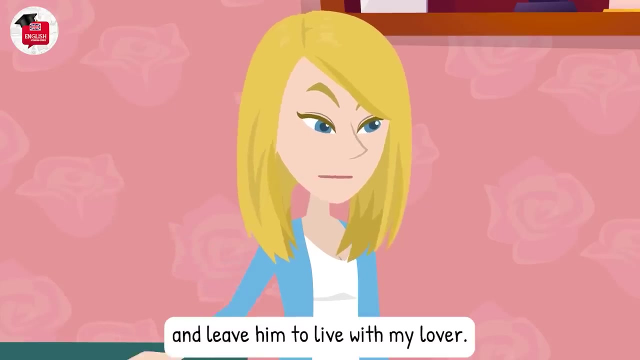 i recognized you. yes, jenny. andrew left you because of me and that stupid kid thought i loved him. you and tony. i just wait for tony to complete his big contract, then i'll find a way to take his money and leave him to live with my lover. i won't let you do that. listen to me, jenny. 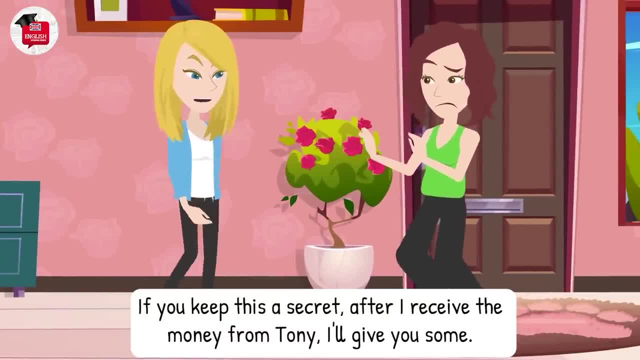 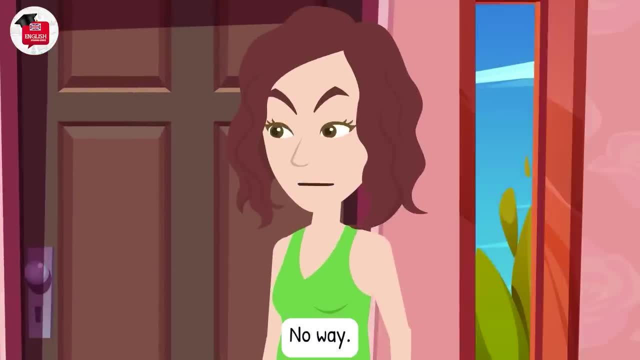 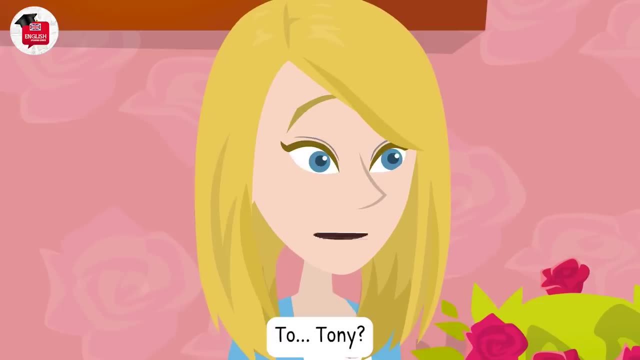 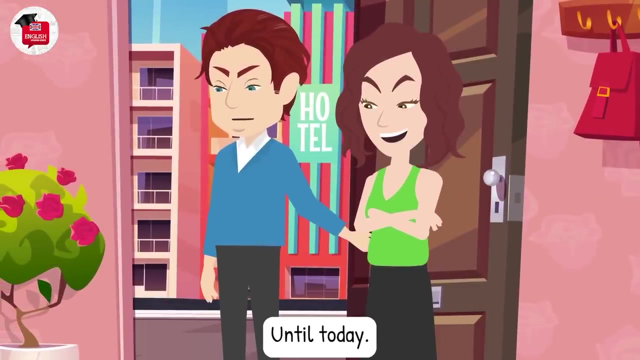 if you keep this a secret, i'm going to kill you. after i receive the money from tony, i'll give you some. you just need to shut up. no way, if you're stubborn, i can make you disappear from tony's life. to tony: jenny told me all about you, but i didn't believe her until today. 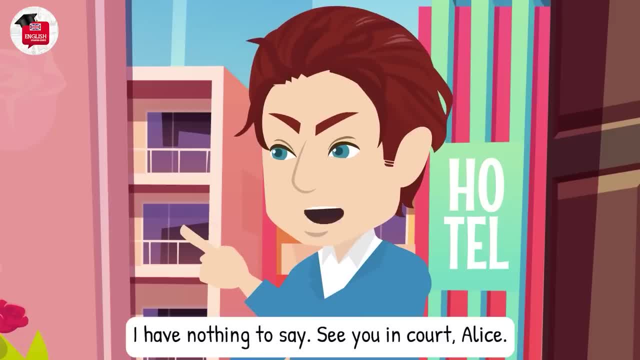 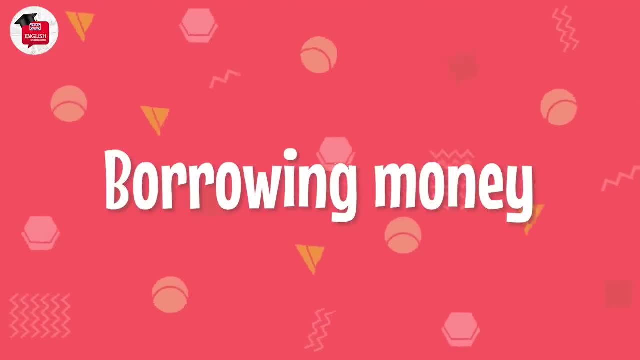 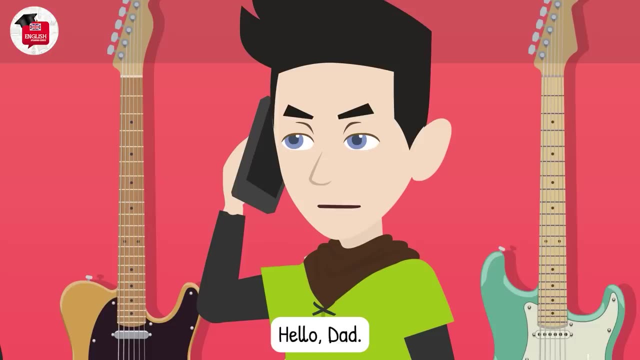 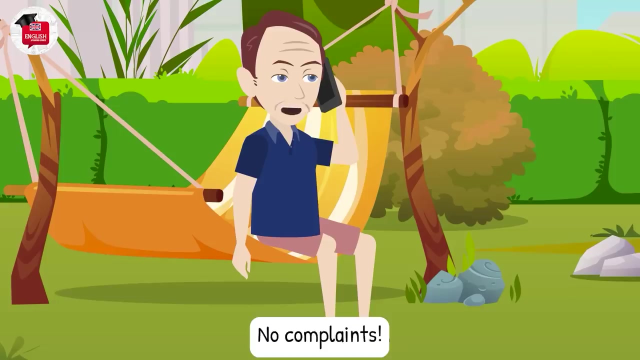 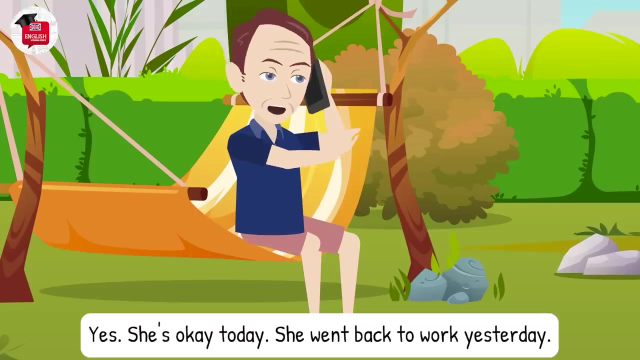 i have nothing to say. see you in court, alice borrowing money. hello, dad, how have you been lately? full of beans and you, no complaints? how's mom? did she get over her cold? yes, she's okay today. she went back to work yesterday. that's great. uh, can you help me, dad? 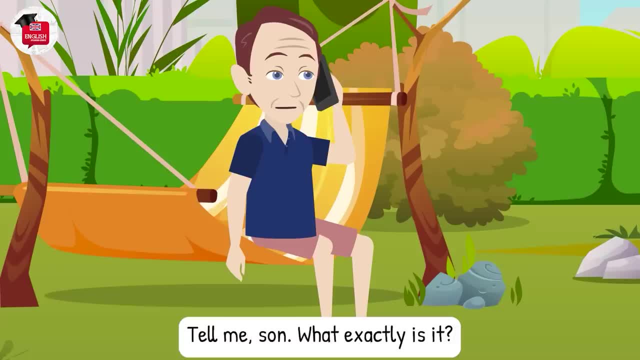 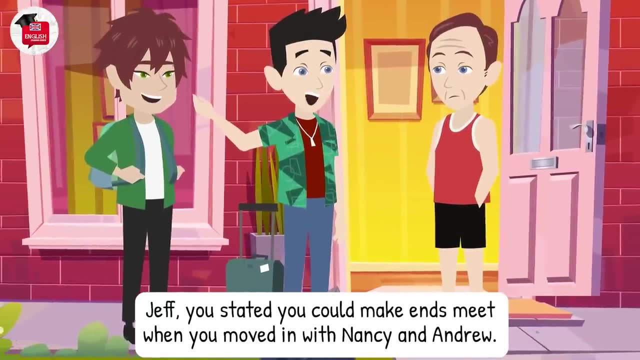 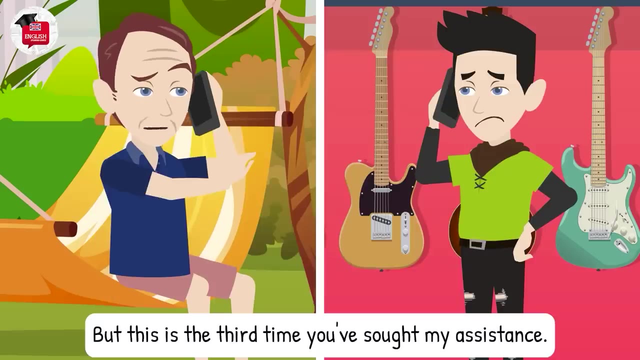 tell me, son, what exactly is it? well, could you just lend me two hundred dollars, jeff? you stated you could make ends meet when you moved in with nancy and andrew, but this is the third time you've sought my assistance. i'm sorry, but my old guitar broke and i had to get a new one. 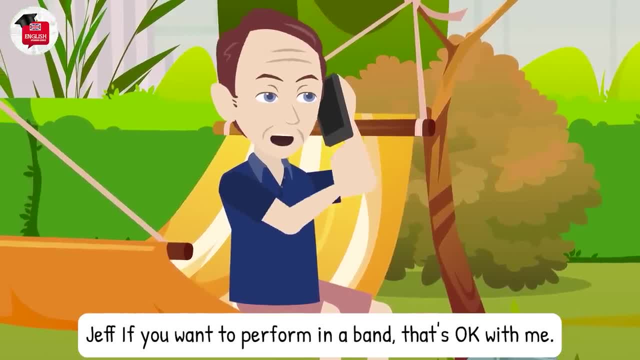 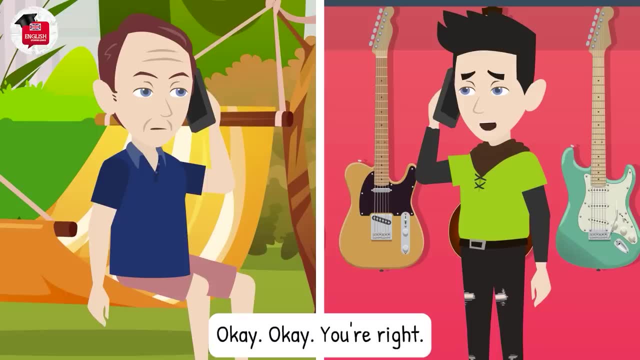 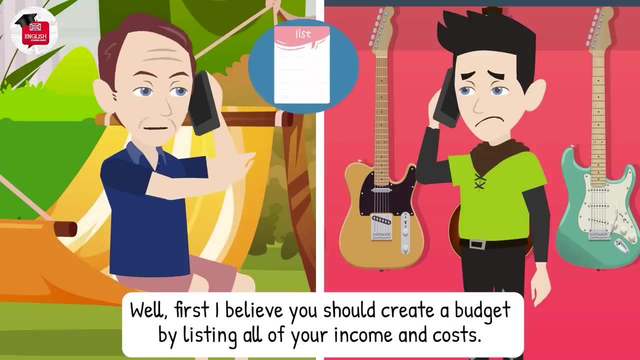 jeff, if you want to perform in a band, that's okay with me, but you can't keep me from doing it. why do you keep asking me to pay for it? okay, okay, you're right. well, first, i believe you should create a budget by listing all of your income and costs. 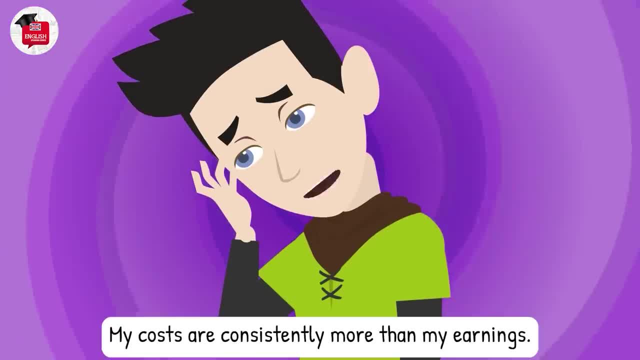 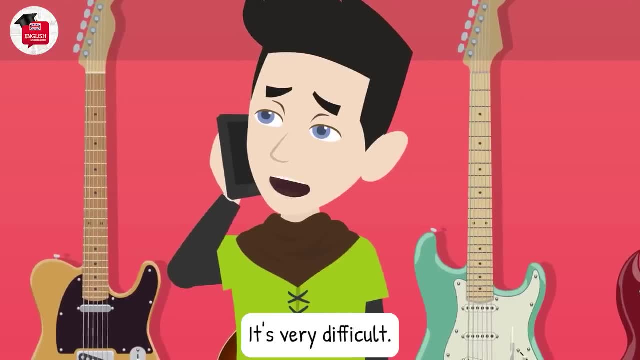 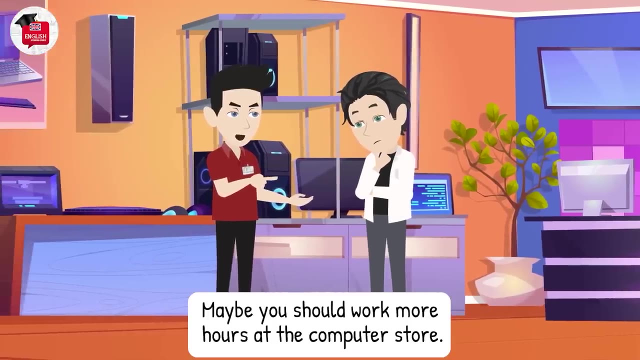 and then it's as simple as not spending more than you earn. my costs are consistently more than my earnings. you should save more. it's very difficult. that's why i need to borrow money from you. then be should work more hours at the computer store. Dad, how can I study and work if I already work? 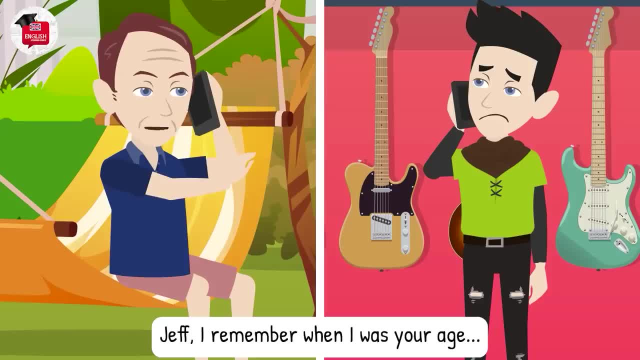 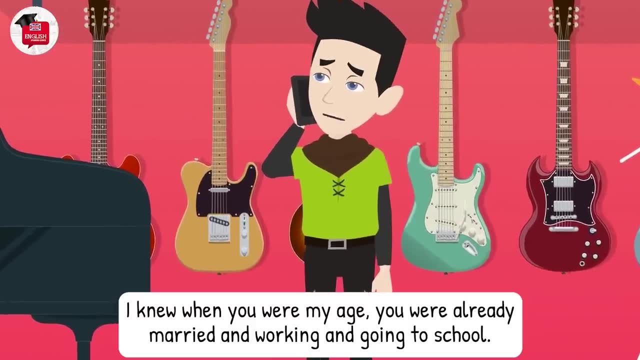 15 hours a week. Jeff, I remember when I was your age. Come on, Dad, I know when you were my age you were already married and working and going to school. That's correct, And if I could do it, 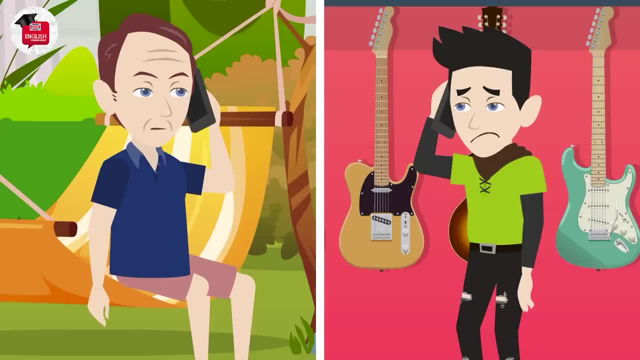 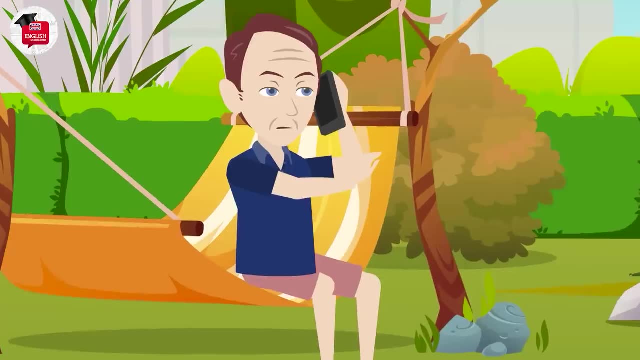 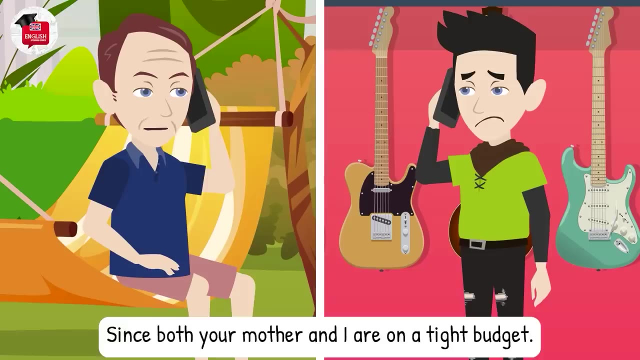 I would. Why can't you Dad? I'm not you, That's why. All right, Jeff, calm down. I don't expect you to be like me, but I can't lend you any more money, since both your mother and I are on a tight budget. Maybe I should just drop out of school, work full time and 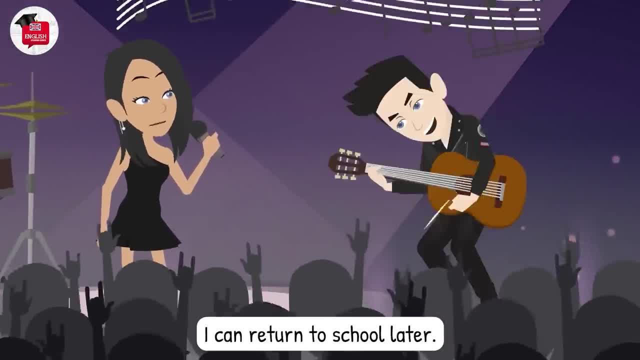 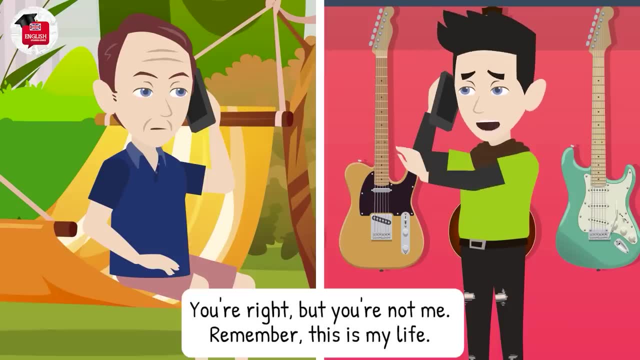 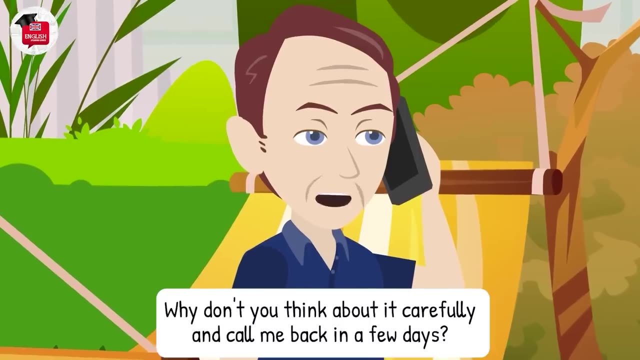 play in the band. in the meanwhile, I can return to school later. If I were you, I would not do so. You're right, but you're not me. Remember: this is my life. Okay then, Let's not debate about it. Why don't you think about it carefully and call me back in? 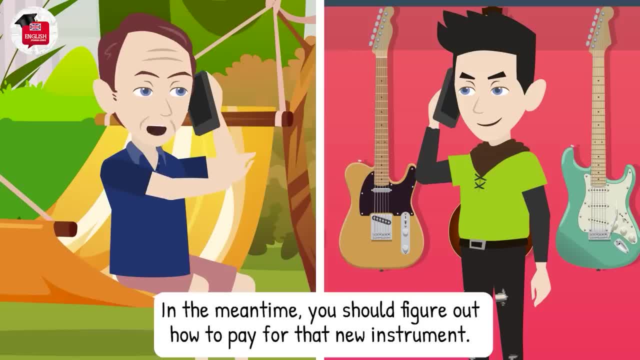 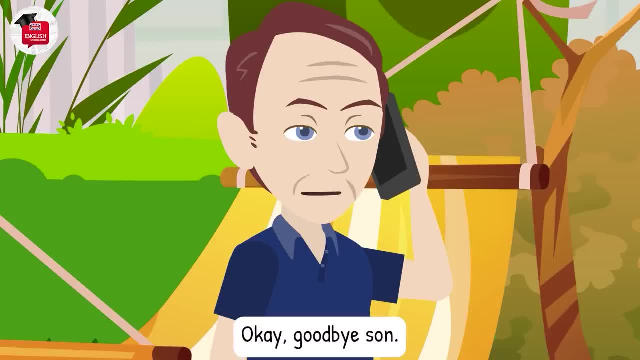 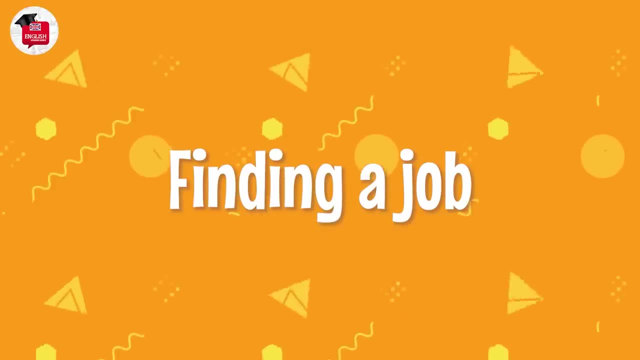 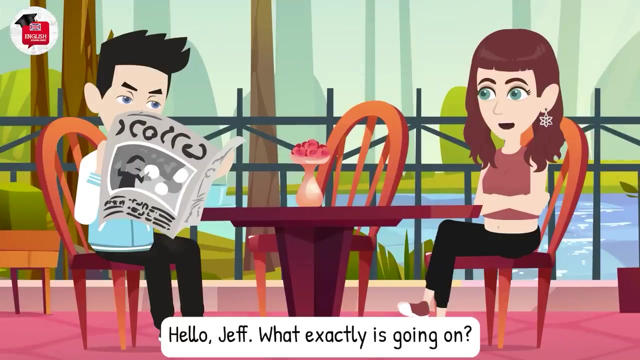 a few days. In the meantime, you should figure out how to pay for that new instrument. Yes, father, Okay, Goodbye son. Finding a Job. Hello Jeff, What exactly is going on? Oh, I'm reading through the classifieds. I guess I'll have to acquire a job. 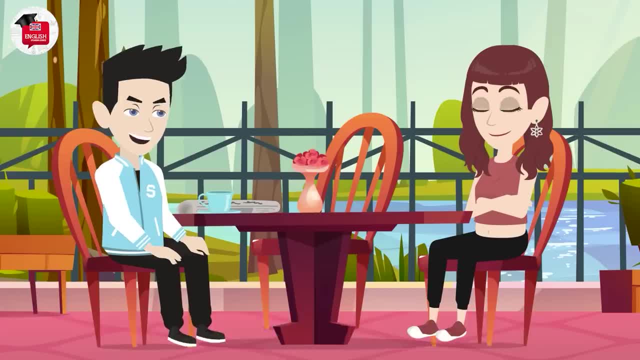 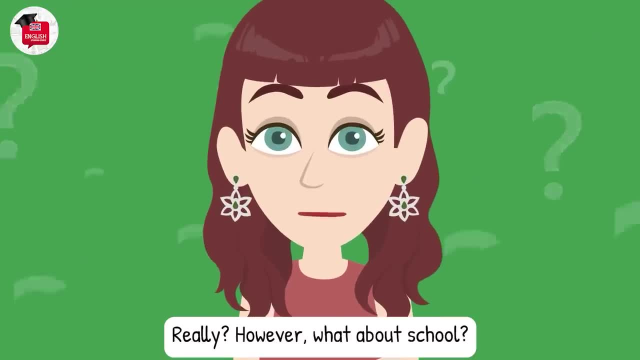 Aren't you working at a computer store or something? Yes, but it is only part time. I need a full time job. What, Really, However? what about school? Well, to tell you the truth, I'm probably going to drop out of school for a while. 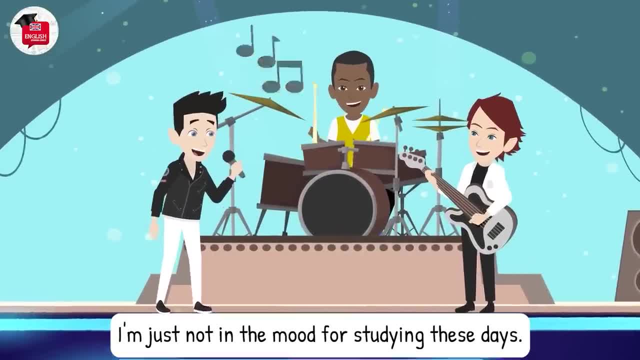 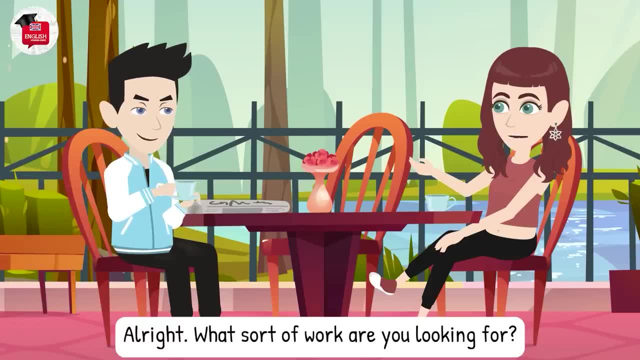 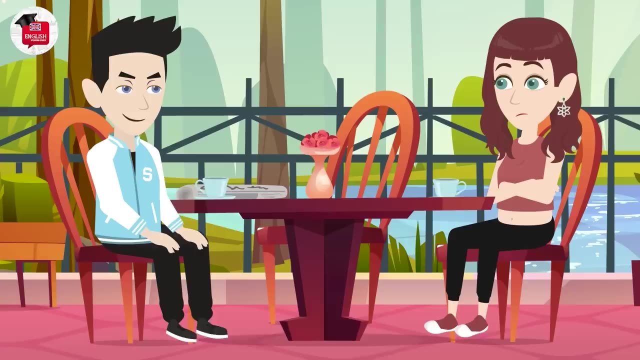 Why I'm just not in the mood for studying these days. I'd rather spend my time playing with my band. Alright, What sort of work are you looking for? Ideally, something involves music, such as in a record shop. Whatever I do, it'll be better than my first job. 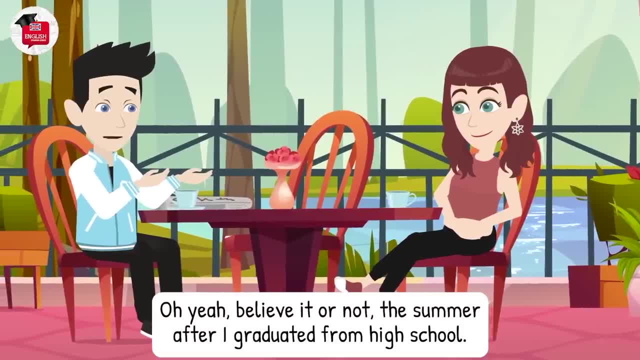 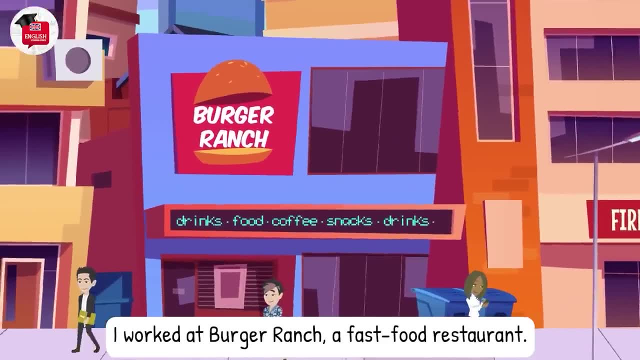 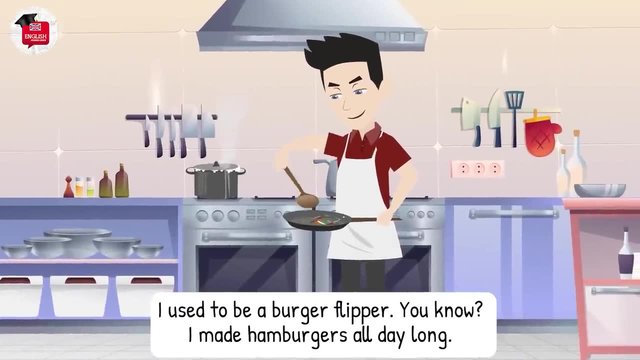 What was your first job? Oh yeah, Believe it or not, the summer after I graduated from high school, I worked at Burger Ranch, a fast food restaurant. What exactly did you do there? I used to be a burger flipper, you know. I made hamburgers all day long. 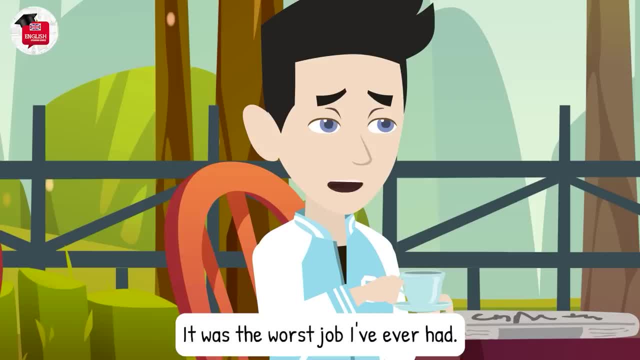 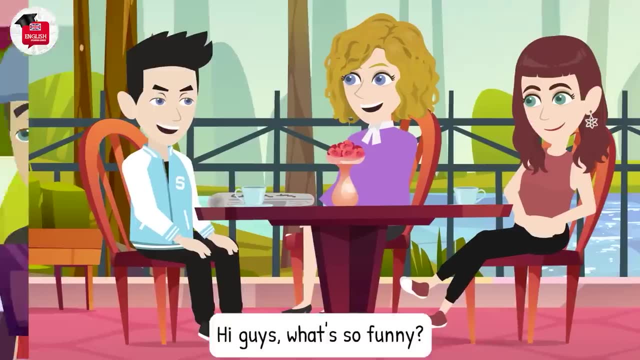 That sounds pretty funny. It was the worst job I've ever had. What's the worst job you've ever had? Hi guys? What's so funny? Oh, hello, Nancy. Do you remember when I worked at the Burger Ranch? 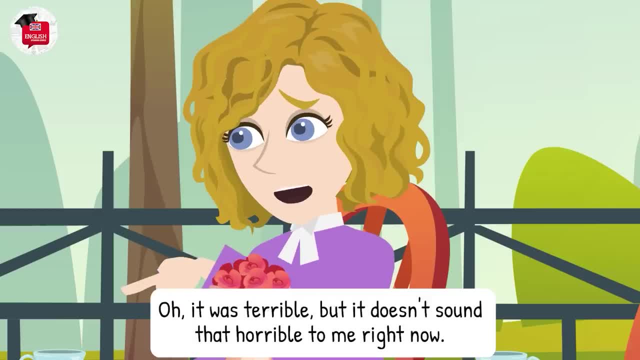 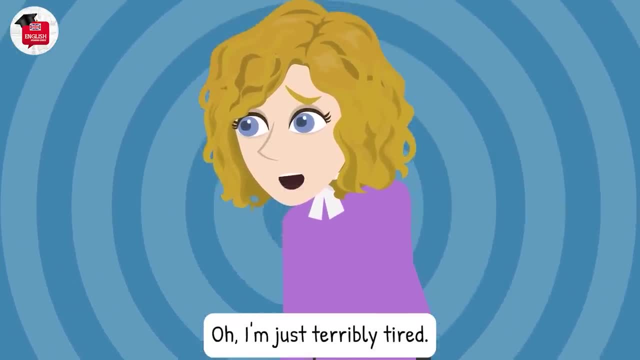 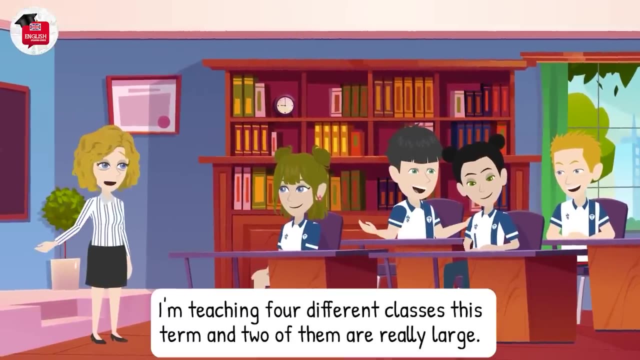 Oh, it was terrible, But it doesn't sound that horrible to me right now. What's the problem? Oh, I'm just terribly tired. What's happened? I'm teaching four different classes this term, and two of them are really large. 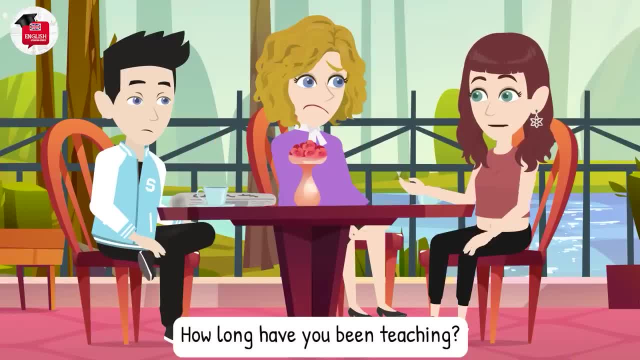 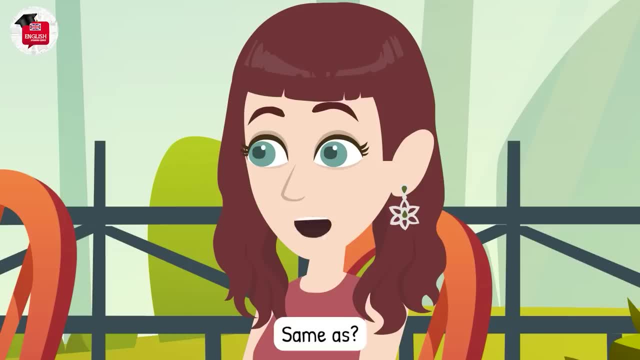 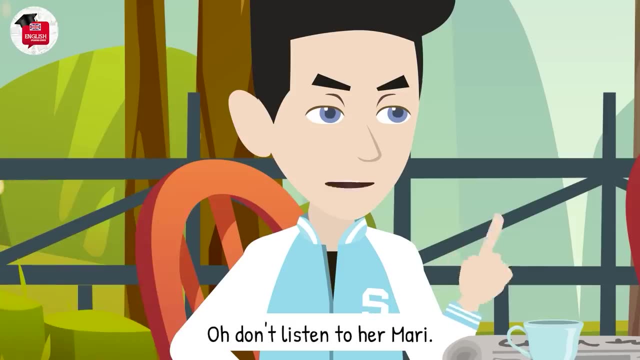 How long have you been teaching? Twelve years. Perhaps it's time to try something new? Same as Well. I've always wanted to be a writer and I could do it from home. Oh, don't listen to her, Mari. 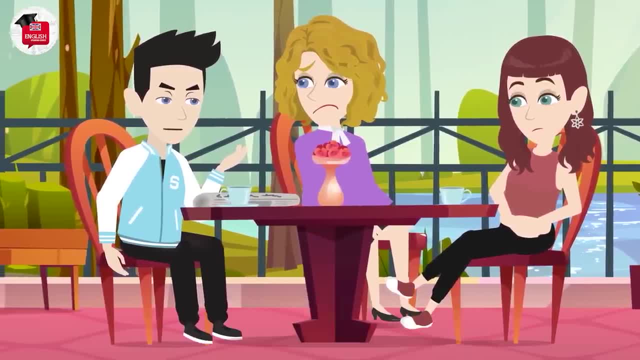 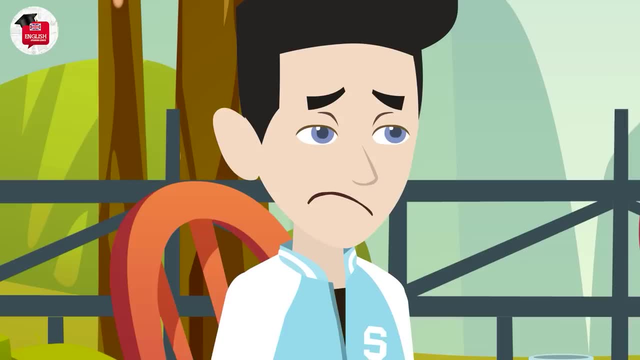 She always talks this way when she's had a bad day at school. At least you have a good job, Nancy. Look at me, Nancy. What's wrong? Hmm, I'm broke And my father will not lend me any more money. 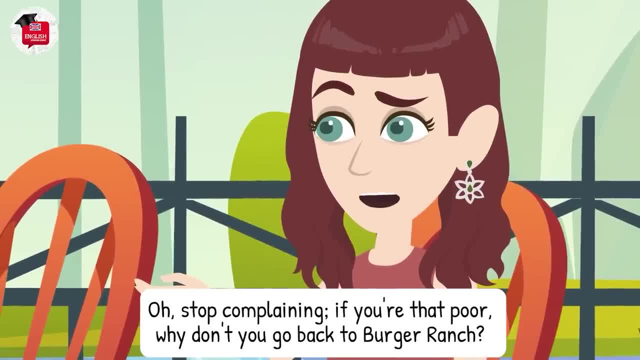 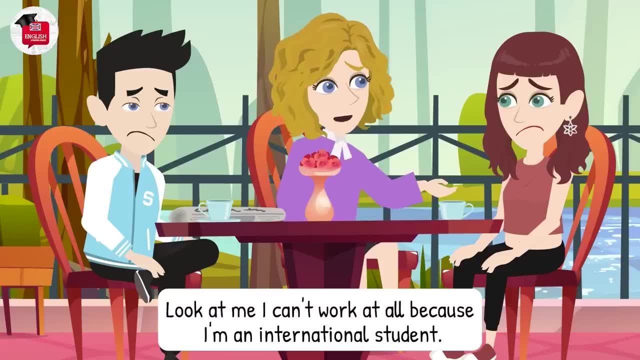 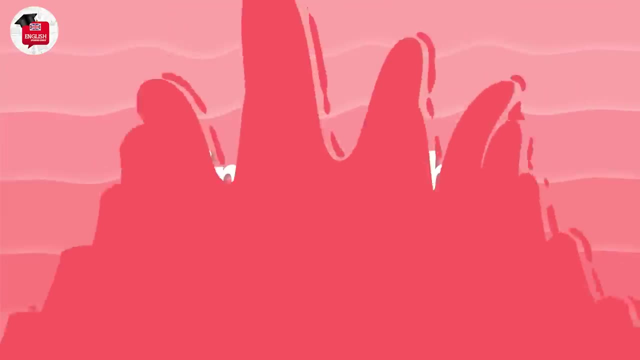 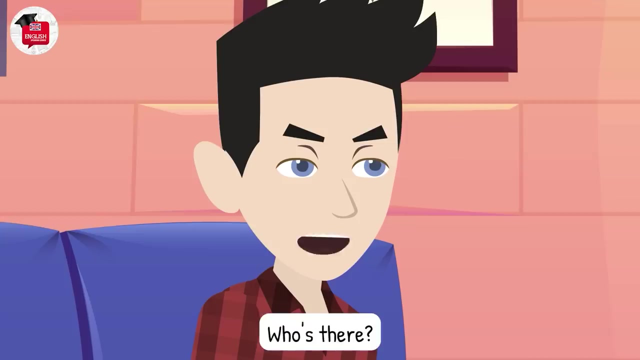 Oh, stop complaining. If you're that poor, why don't you go back to Burger Ranch? Listen, stop arguing. Look at me. I can't work at all because I'm an international student, A single mother Who's there? 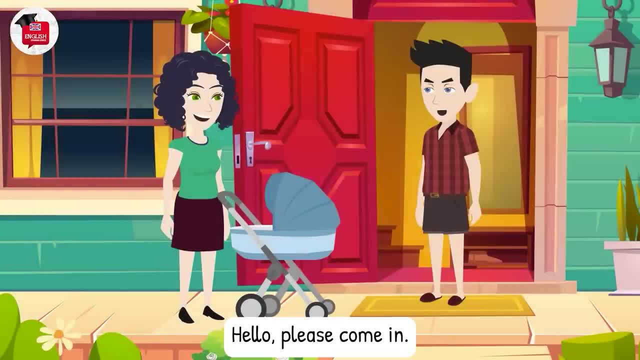 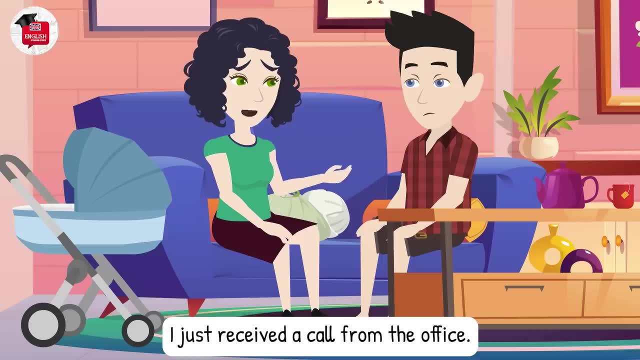 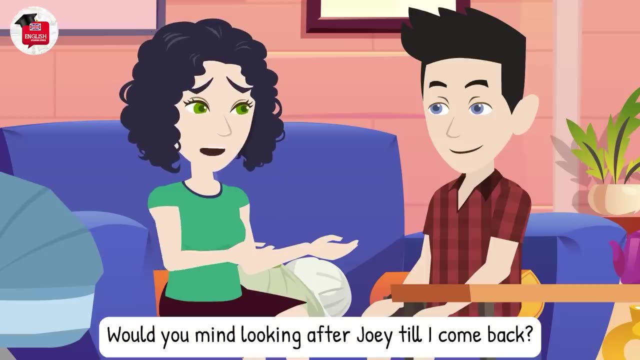 It's Sharon and Joey. Hello, Please come in, Jeff, could you do me a favor? Yes, tell me. I just received a call from the office. They want me to look at a computer problem as soon as possible. Would you mind looking after Joey till I come back? 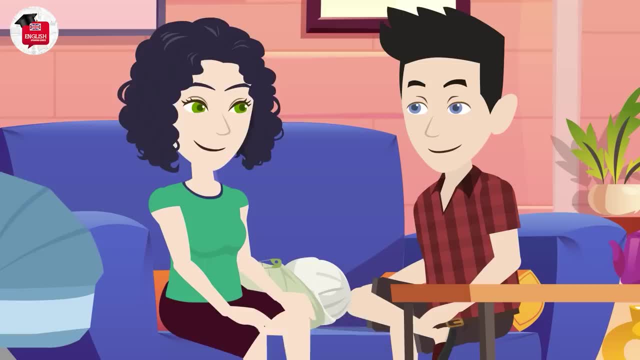 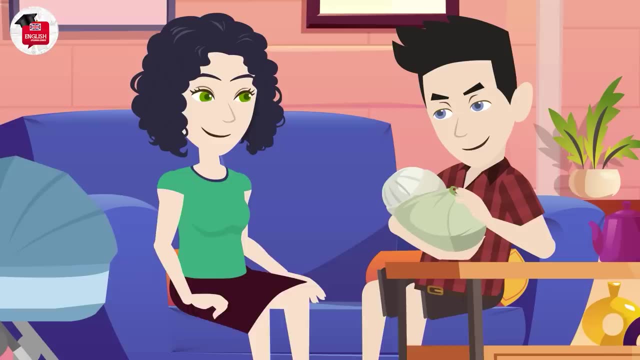 Sure, no worries. Is he sleeping? Yes, he fell asleep five minutes ago At this time, At this time of day. he normally sleeps for a couple of hours, But if he wakes up, simply give him a bottle. What a sweet baby. 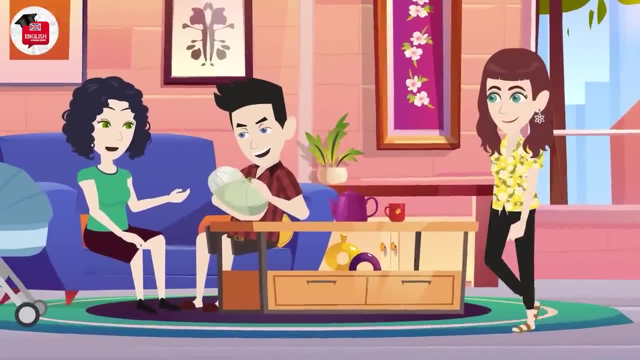 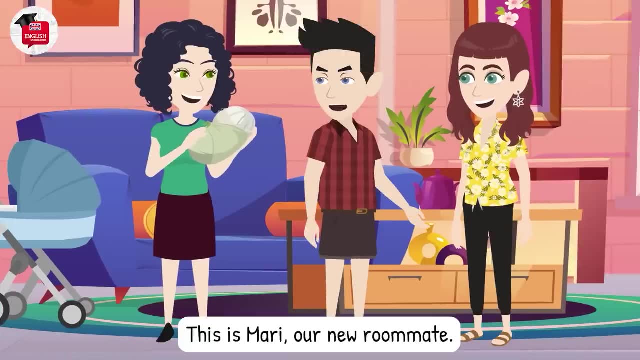 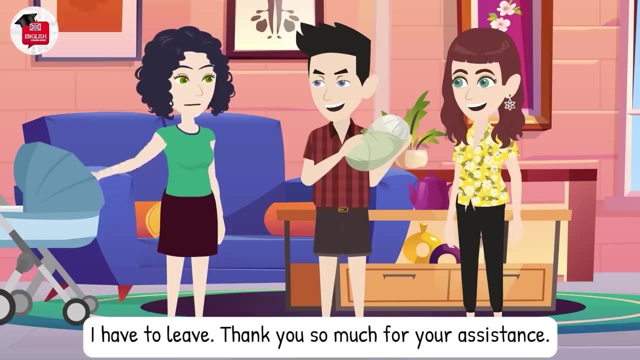 He's so little. This is our neighbor Sharon And her son Joey. This is Mari, our new roommate. Mari, it's a pleasure to meet you. Glad to see you. I have to leave. Thank you so much for your assistance. 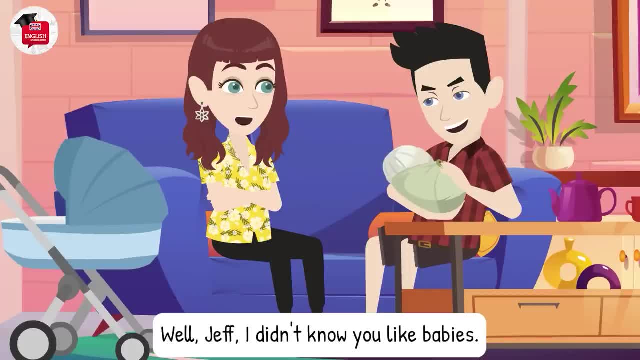 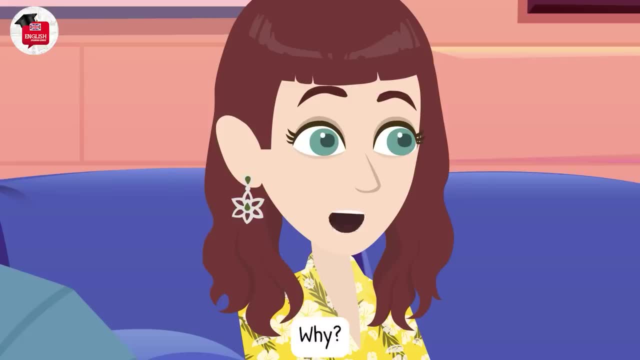 You're welcome. You're welcome, You're welcome. Whoa, Jeff, I didn't know you like babies. Well, Joey is special. Why? Because the baby is so cute And she always lends me her car when I need. 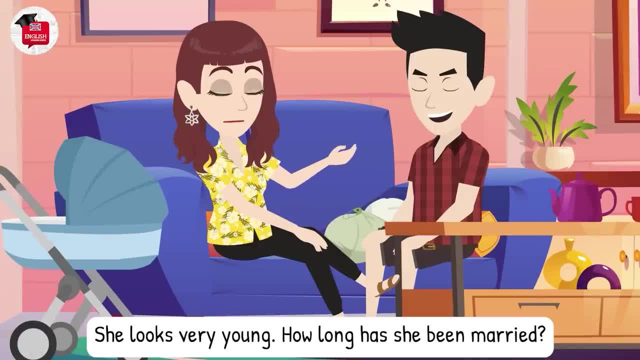 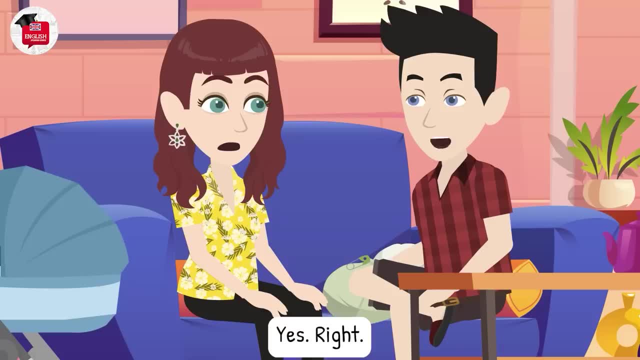 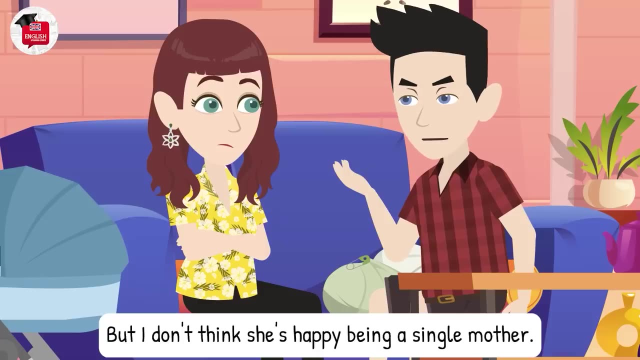 She looks very young. How long has she been married? She is unmarried. Really, Is she a single mother? Yes, right, Is she happy? I don't know, But I don't think she's happy being a single mother. Oh, is that pretty common in America? well, 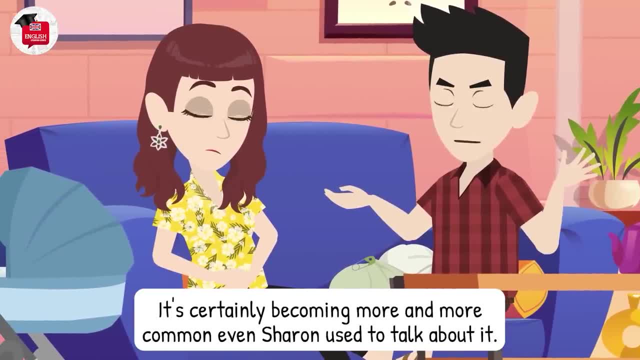 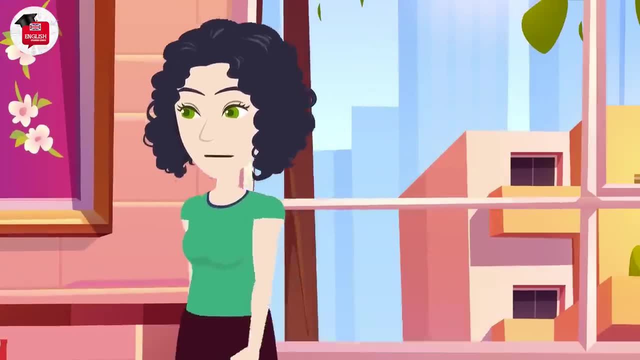 It's certainly becoming more and more common. Even Sharon used to talk about it, You know, before she got married. Hello, what were you saying about me? Oh, hello, That you used to talk about having a baby by yourself before you met Andrew. 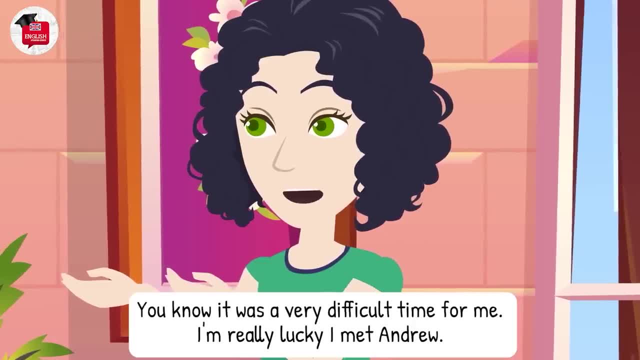 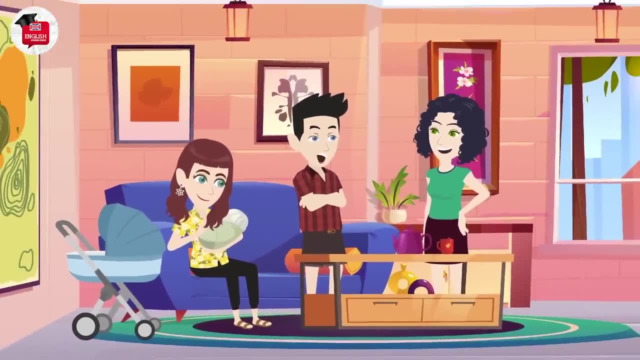 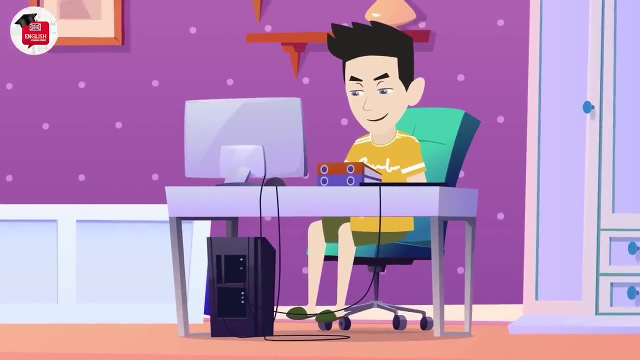 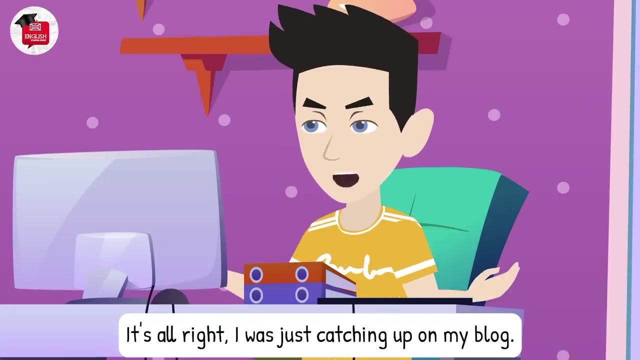 Oh yeah, You know it was a very difficult time for me. I'm really lucky I met Andrew. Cell phone bill: Is it okay if I come in? It's alright? I was just catching up on my blog. Oh, yes, What is your blog about? 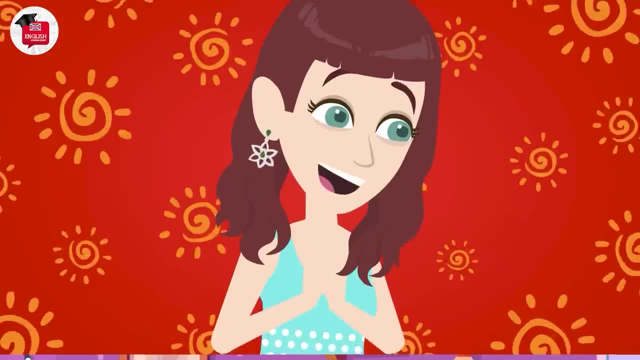 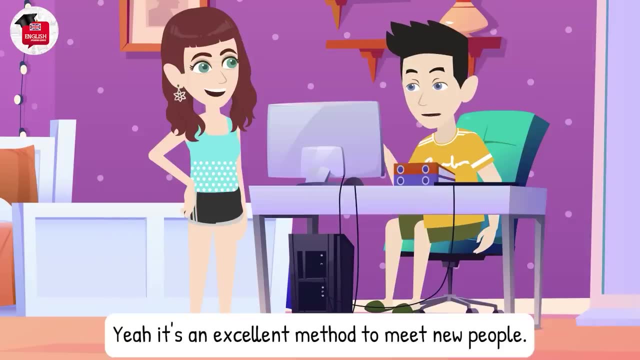 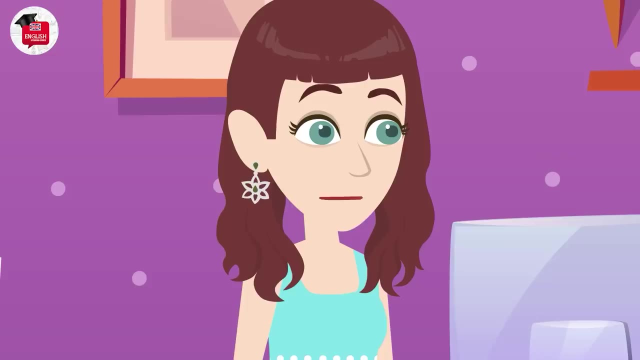 Mostly about hip-hop. Oh, that's great. What are the benefits of blogging? Yeah, it's an excellent method to meet new people, Really. Yeah, you make friends with people you wouldn't have met otherwise. Perhaps I should create a blog in English learning. 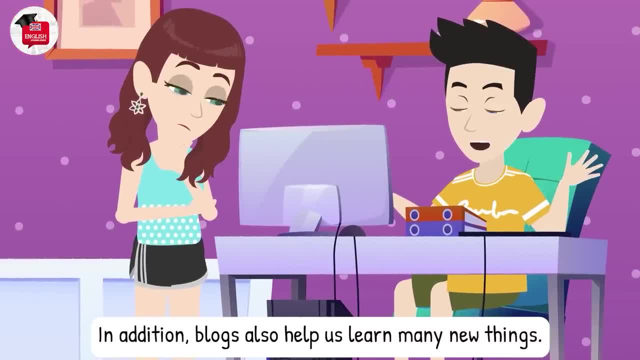 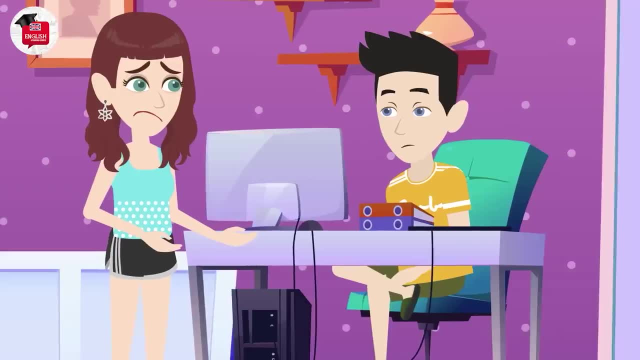 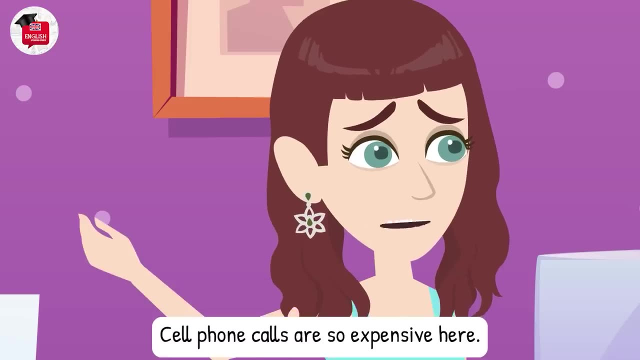 In addition, blogs also help us learn many new things. I know I wanted to ask your advice. Yeah, Yes, tell me. Well, I just got my cell phone bill for last month and it was $160.. Cell phone calls are so expensive here. 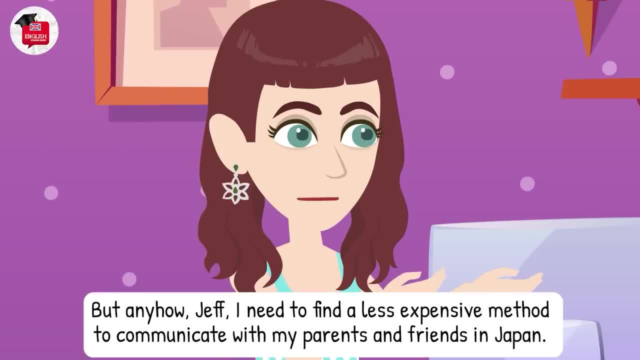 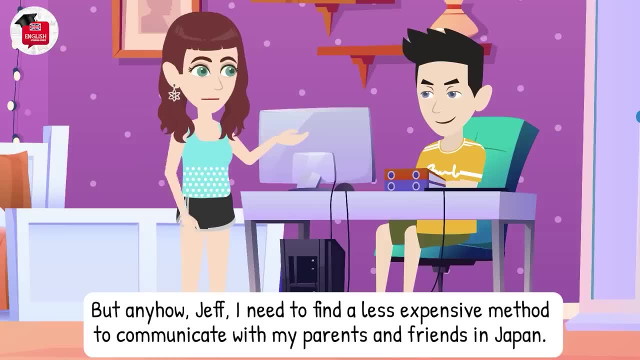 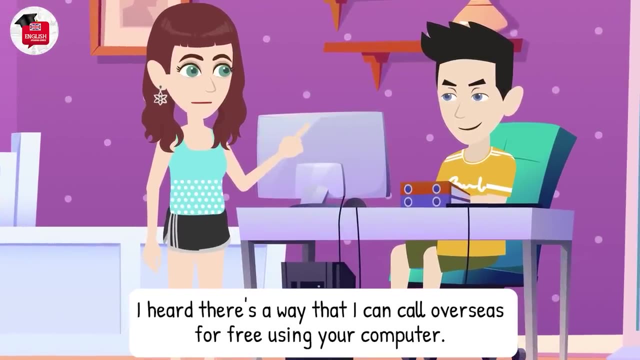 Yeah, so expensive. But anyhow, Jeff, I need to find a less expensive method to communicate with my parents and friends in Japan. Please go ahead. I heard there's a way that I can call overseas for free using your computer. Do you know anything about that? 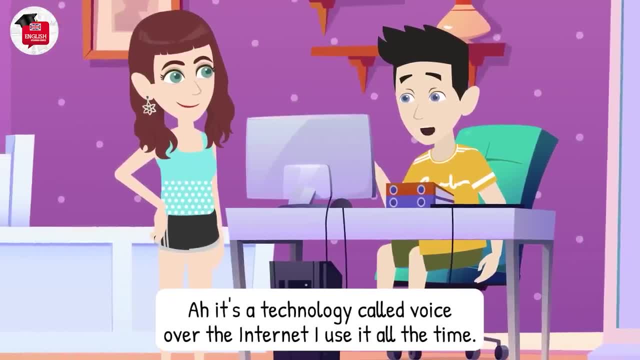 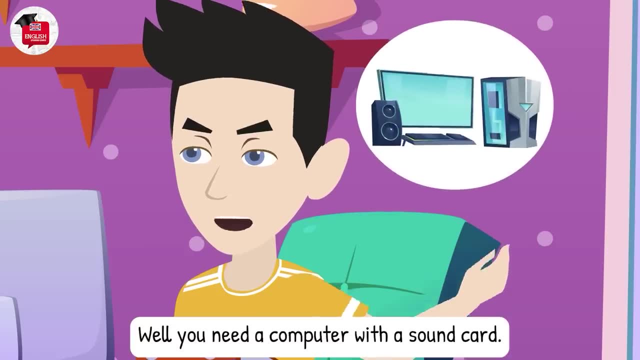 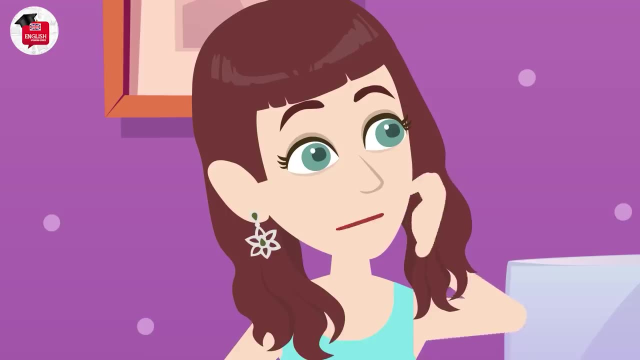 Ah, it's a technology called voice over the internet. I use it all the time. How does it function? Well, you need a computer with a sound card. Yes, I do. You also need a microphone and a headset. I don't have any of those. 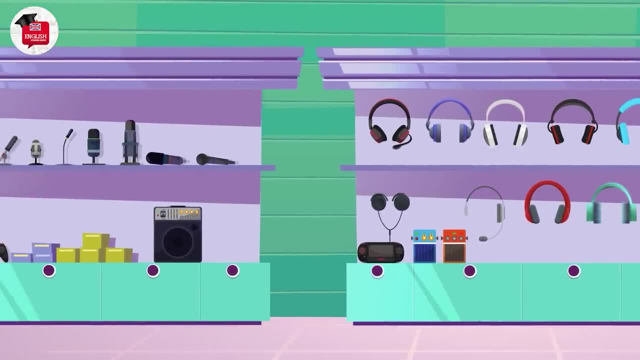 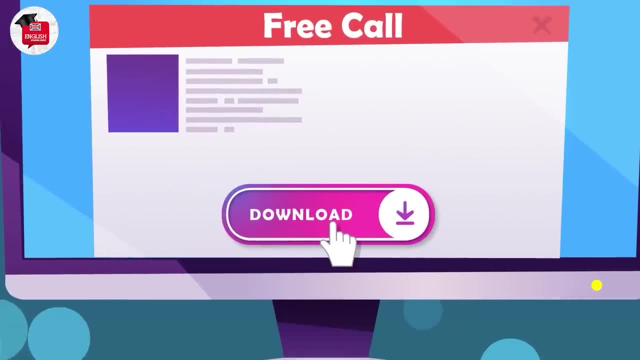 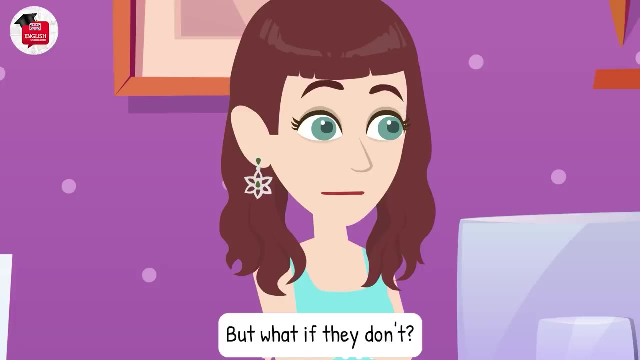 You can get these at any electronic store. Anything else, No, I don't have any of those. Then you'll need to download the program which is free and then hope that the person you're calling downloads the same software which allows you to call for free. 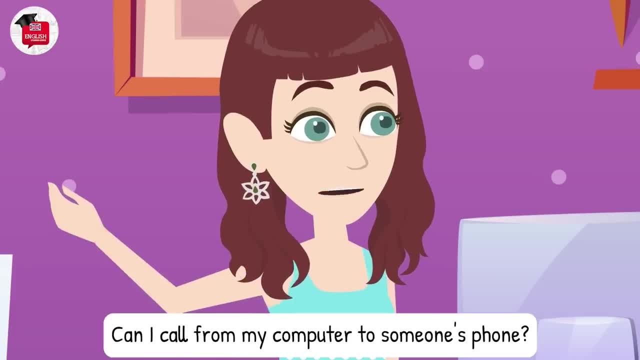 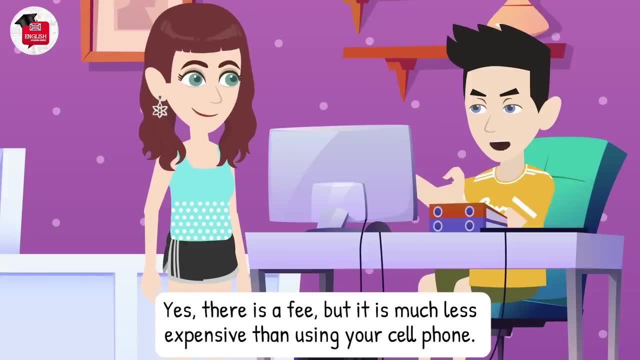 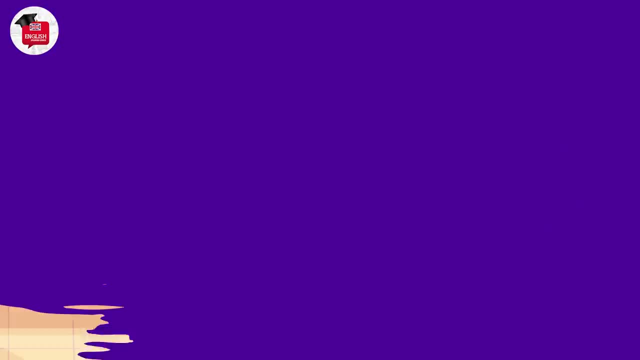 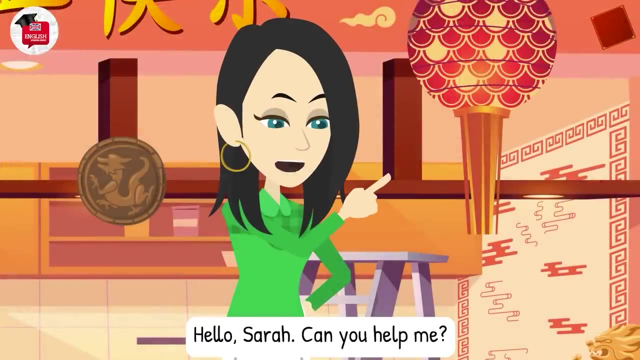 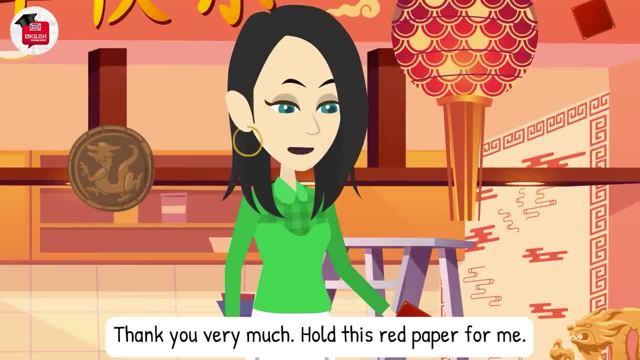 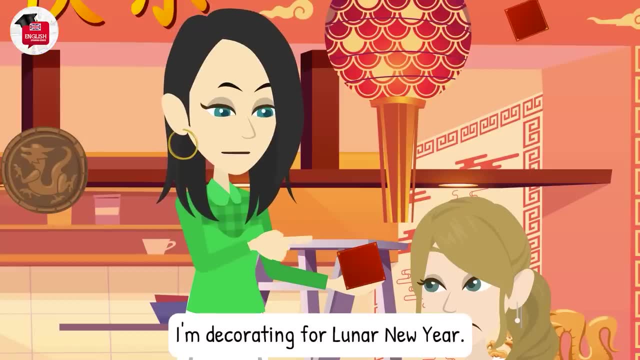 Sure, What do I have to do now? Thank you very much. Hold this red paper for me, OK. What exactly are you doing now? I'm decorating for Lunar New Year. I don't know too much about Lunar New Year. What's a call to Lunar New Year? 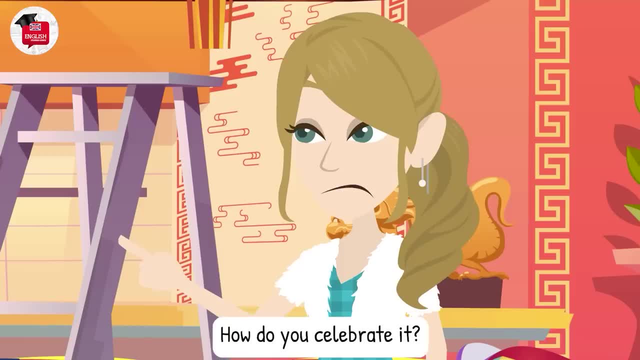 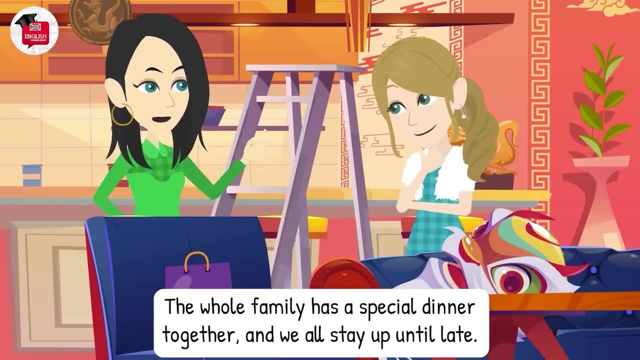 as the dates of celebration follow the phases of the moon. How do you celebrate it? Family gathers together on Lunar New Year's Eve. The whole family has a special dinner together and we all stay up until late. What do you eat? We eat chicken, fish, noodles and dumplings. 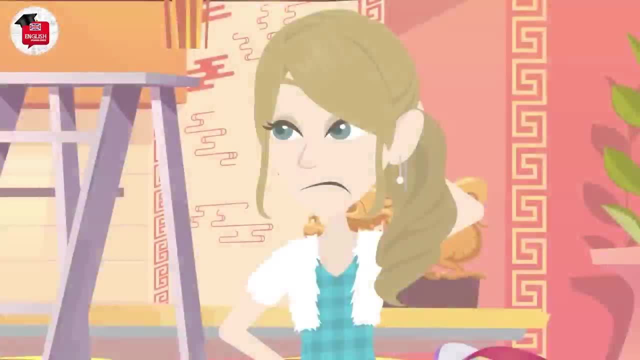 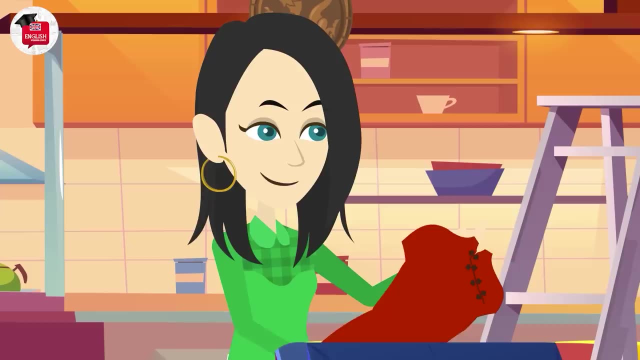 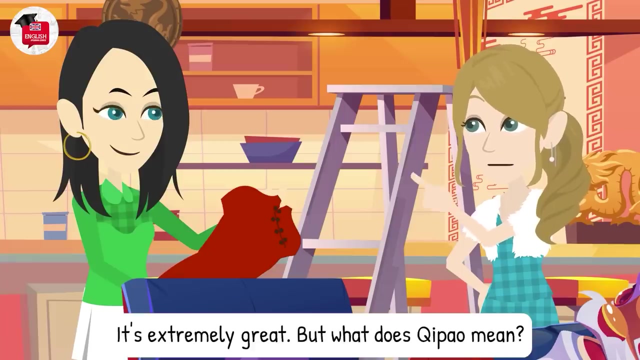 And parents gift their kids red envelopes. What are red envelopes? The envelopes have money inside. Oh, cool. Hey, Sarah, take a look at my qipao. It's extremely great. but what does qipao mean? A type of dress traditionally worn by Chinese women. 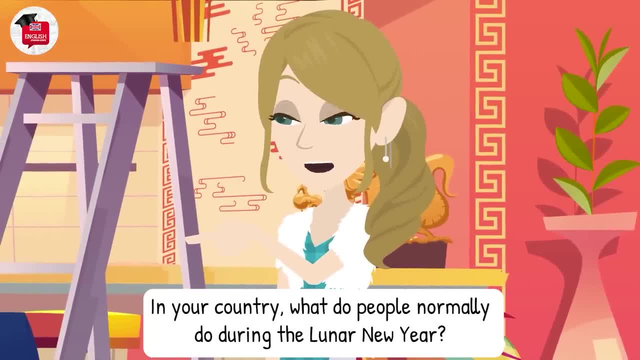 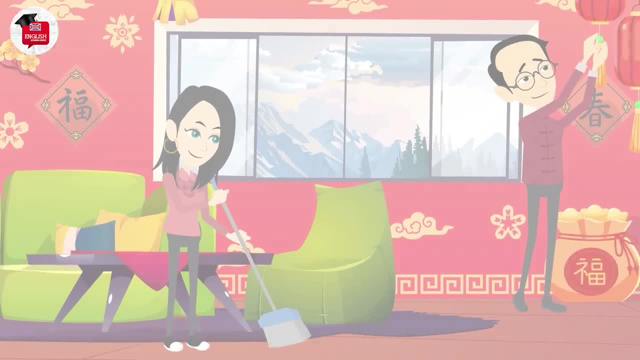 Great. In your country, what do people normally do during the Lunar New Year? A few days before the New Year, we clean the house and decorate the walls with red paper. Lunar New Year sounds interesting. I can write about it for the newspaper. 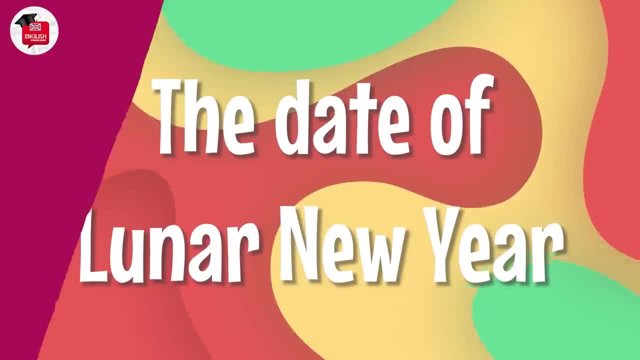 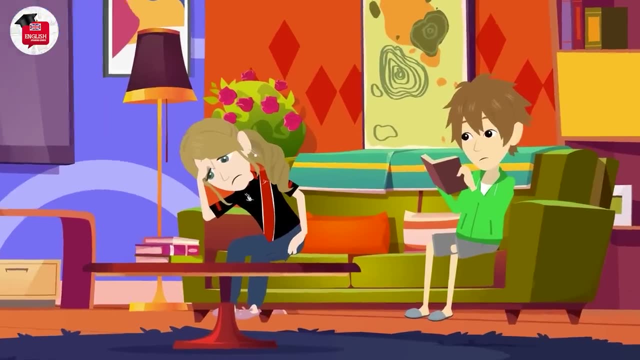 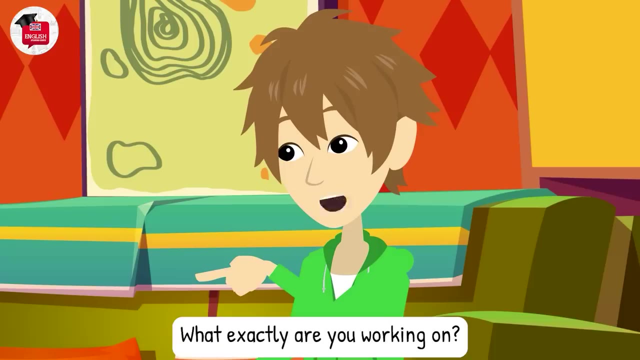 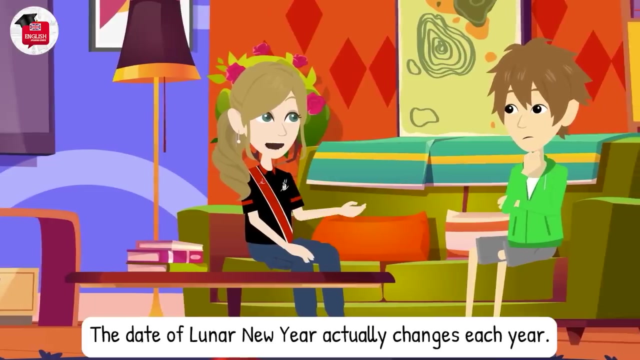 The date of Lunar New Year. The date of Lunar New Year? Ugh, I have a lot of work to do. What exactly are you working on? I'm writing a column about Lunar New Year. Great, The date of Lunar New Year actually changes each year. 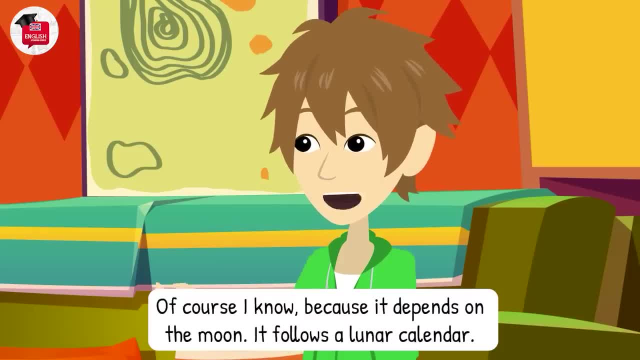 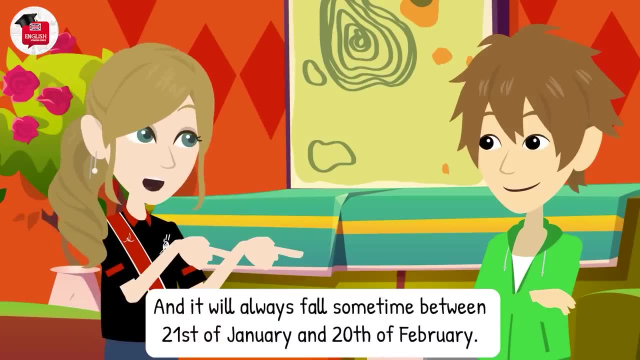 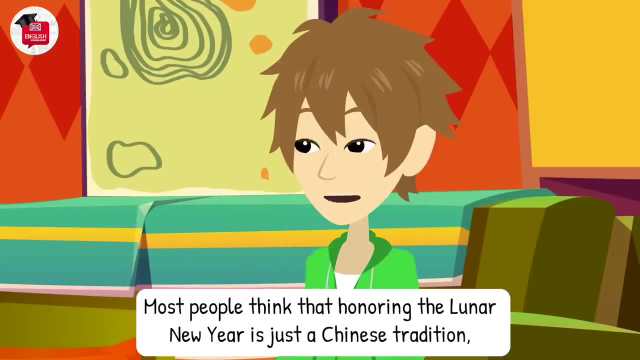 Did you know that? Of course I know, Because it depends on the moon. it follows the lunar calendar, That's correct, And it will always fall sometime between 21st of January and 20th of February. Most people think that it's honoring the Lunar New Year is just a Chinese tradition. 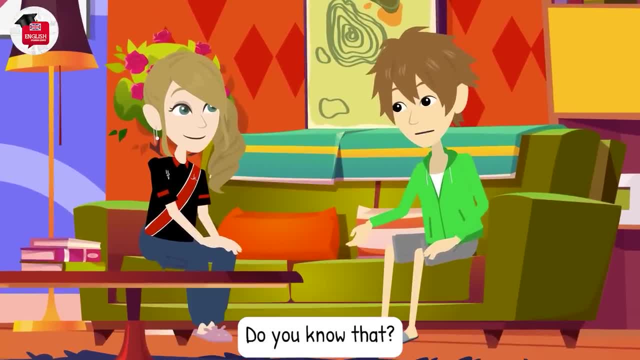 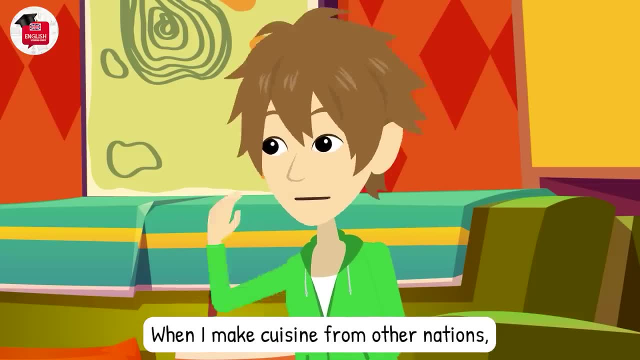 But it's an event that's been celebrated in many countries in Asia. Do you know that? Yes, Mark, how do you know all this? When I make cuisine from other nations, I try to learn about their cultures as well. I like learning about different cultures and delicacies. 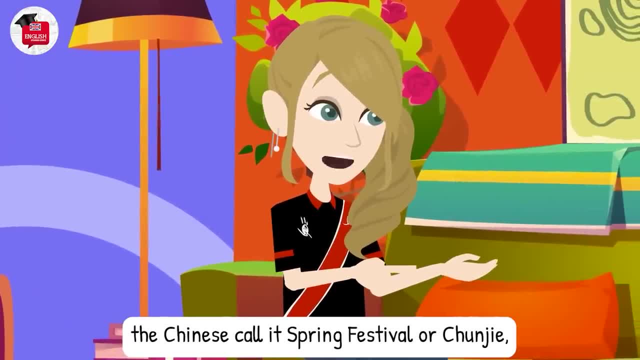 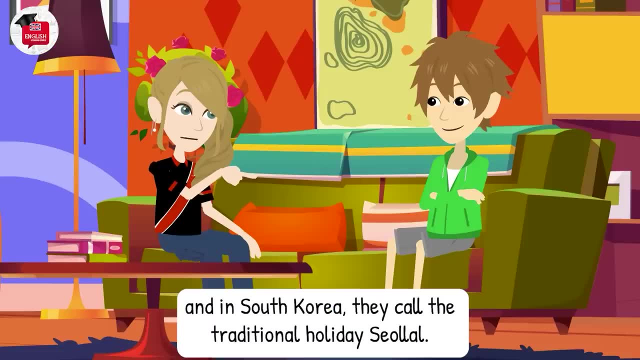 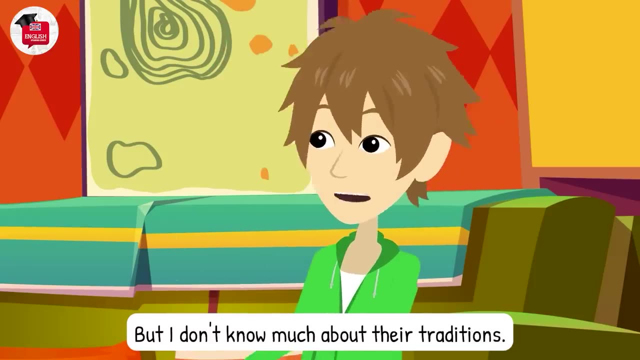 Cool. Although the Chinese New Year is celebrated in winter, the Chinese call it Spring Festival, or Chunchi, And in South Korea they call the traditional holiday Solal, And in Vietnam they call it Dat Nguyen Dan, But I don't know much about their traditions. 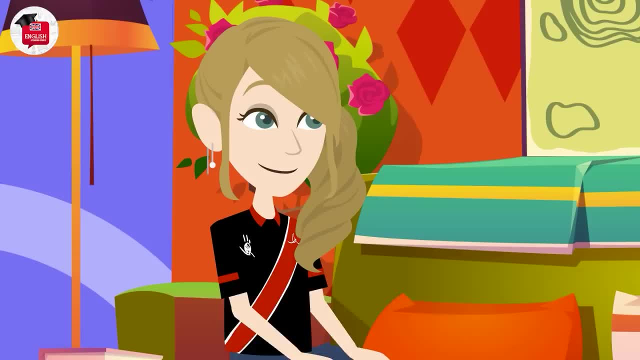 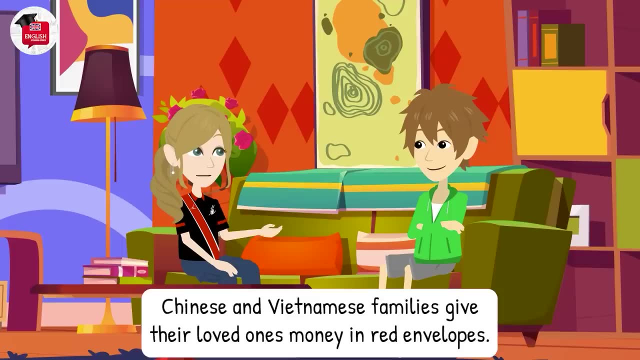 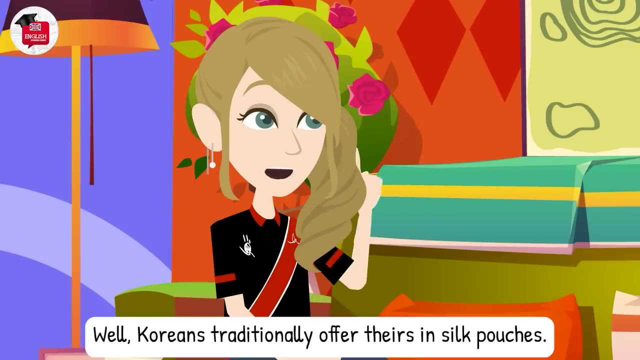 I know some traditions. Tell me, Despite the difference in names, they have similar traditions. Fantastic. Tell me more. Chinese and Vietnamese families give their loved ones money in red envelopes, While Koreans traditionally offer theirs in silk pouches. Whoa, anything else? 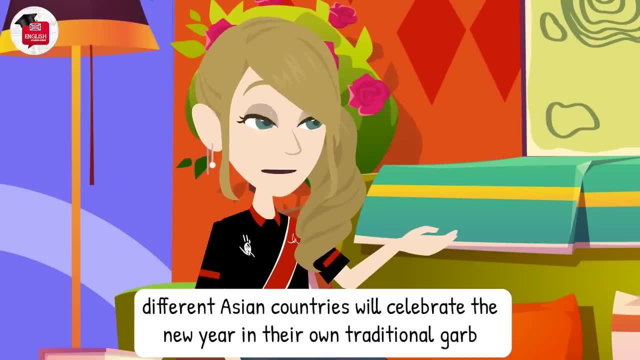 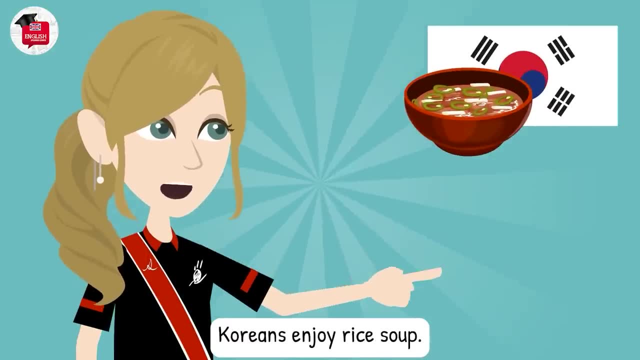 And, of course, different Asian countries will celebrate the New Year in their own traditional garb. What about food? The food is different. Koreans enjoy rice cake soup. Vietnamese eat rice cake soup. Vietnamese eat rice cake soup. Well, I want to try to make that. 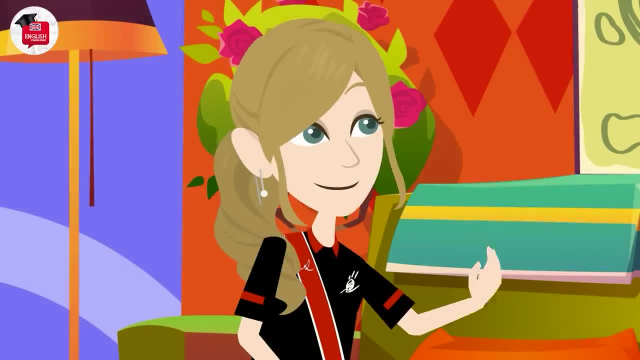 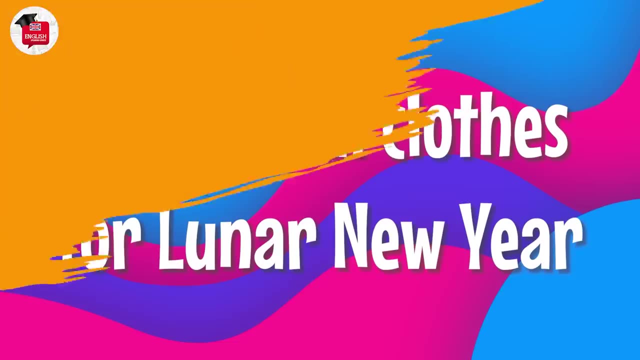 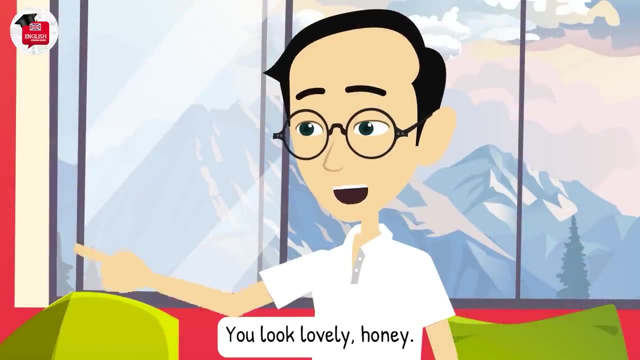 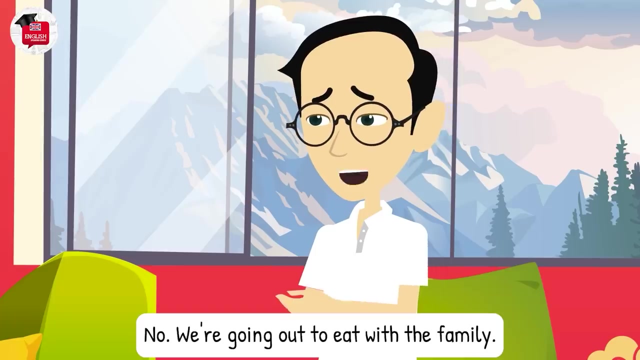 I'll cook some New Year's food for us. Traditional clothes for Lunar New Year. You look lovely, honey. Thanks, But why are you wearing shorts Tonight's Lunar New Year's Eve, Did you forget? No, We're going out to eat with you. 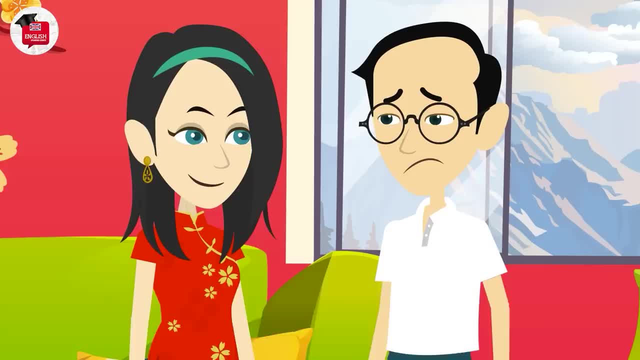 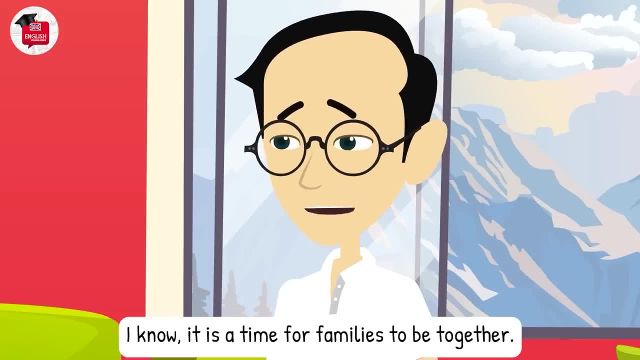 With the family. But, honey, I don't want to go. Honey, you know, Lunar, New Year's Eve is the most important time, I know. It is a time for families to be together. So we have to go change your clothes. 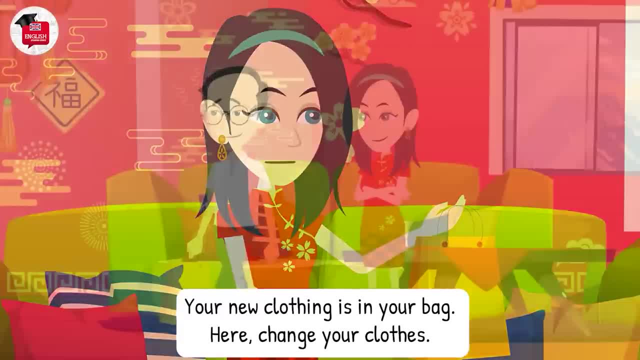 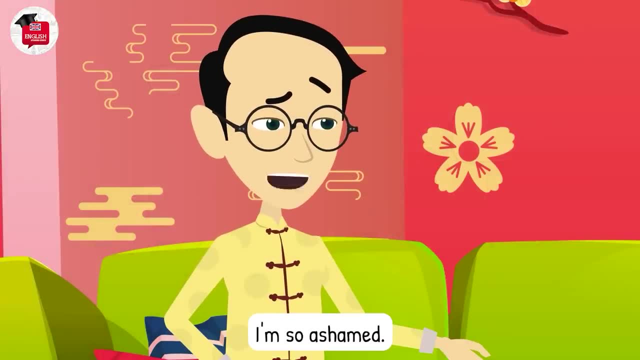 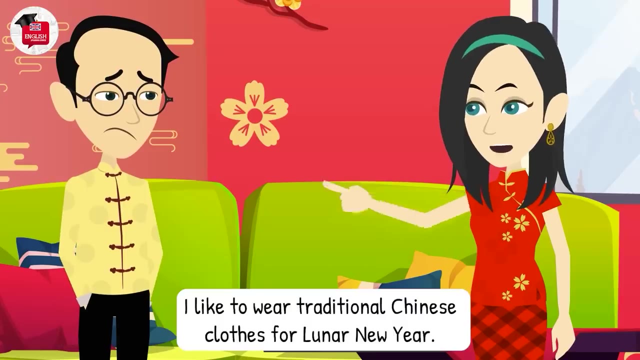 Your new clothing is in your bag Here. change your clothes. Why should I wear this, honey? I'm so ashamed. Why I feel silly? I like to wear traditional Chinese clothes for Lunar New Year. We'll be a hit at dinner. 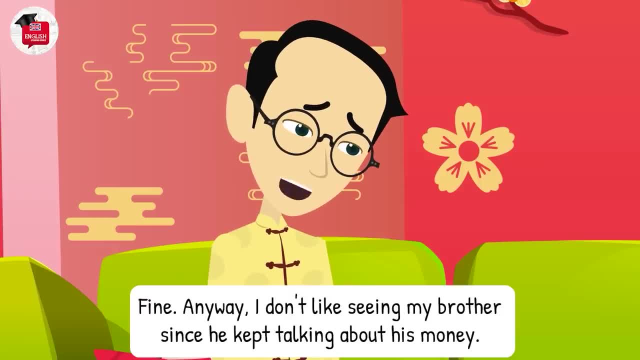 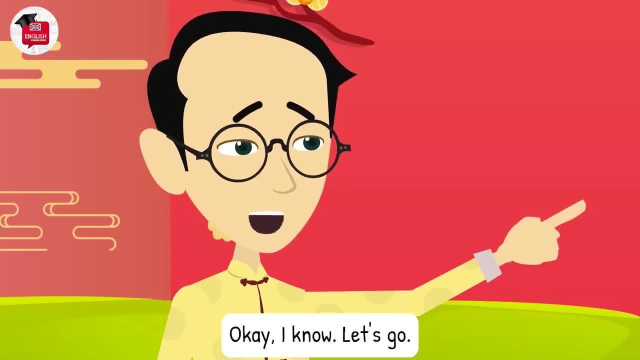 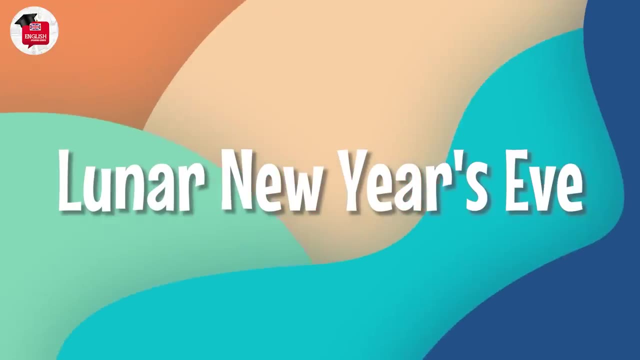 Fine. Anyway, I don't like seeing my brother, since he kept talking about his money, I know, But he's a member of the family. Okay, I know, Let's go. Happy Lunar New Year. Lunar New Year's Eve. 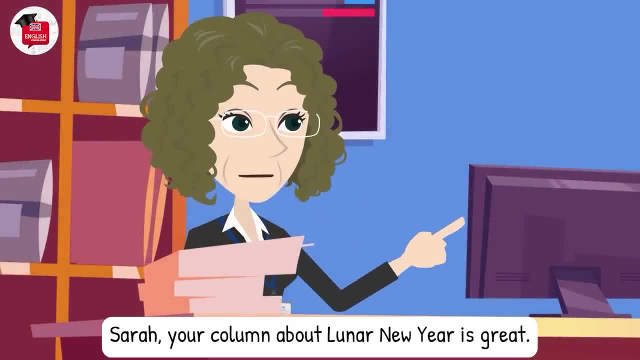 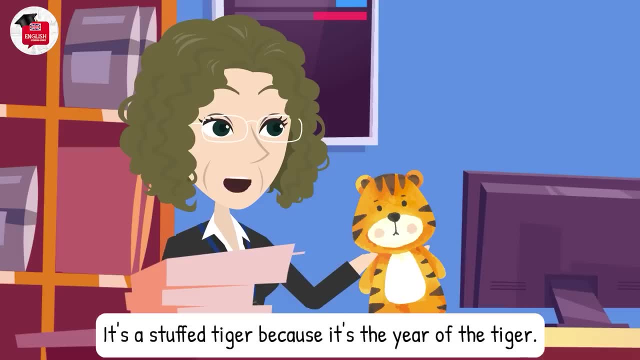 Sarah, your column about Lunar New Year is great. I think you are a great writer. Thank you, And I have a present for you. It's a stuffed tiger because it's the year of the tiger. Thanks, I also have a present for you. 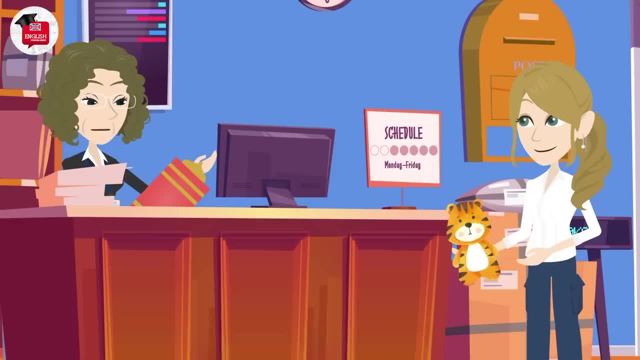 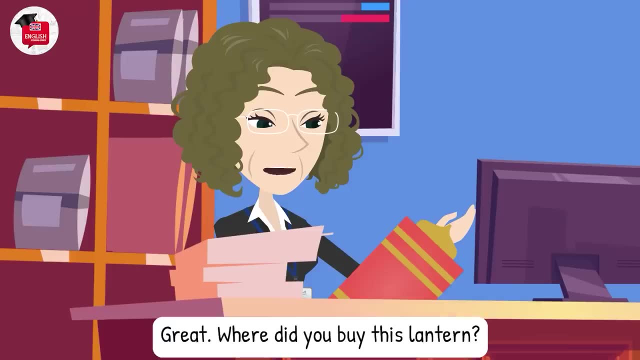 Thanks. What exactly is it? It's a paper lantern from China. It's flat now, but when you pick up the top it opens up. It's flat now, but when you pick up the top it opens up. Great, Where did you buy this lantern? 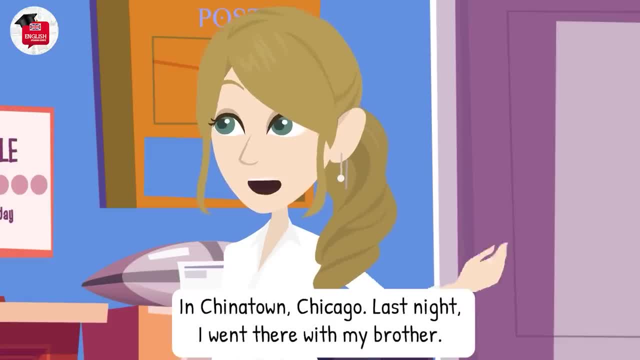 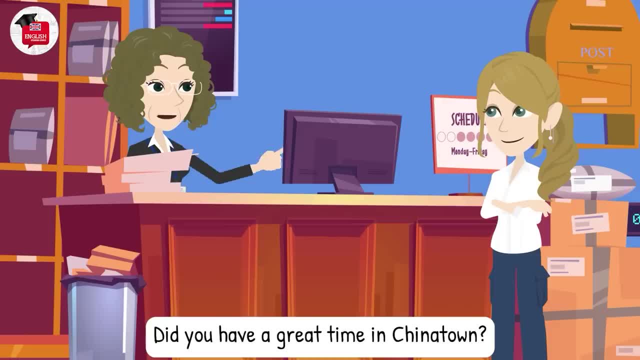 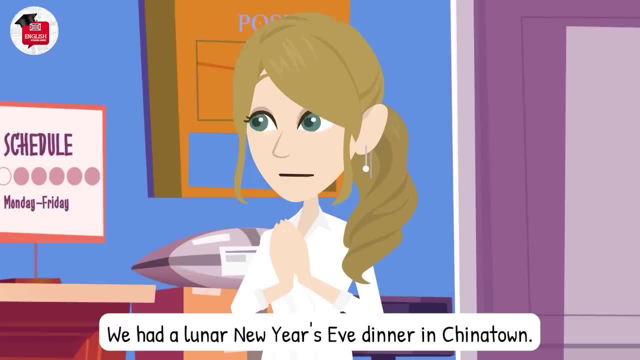 Well, we spent two hours driving the car. Well, we spent two hours driving the car. Did you have a great time in Chinatown? Sure, we had fun. We had a Lunar New Year's Eve dinner in Chinatown. We had a Lunar New Year's Eve dinner in Chinatown. 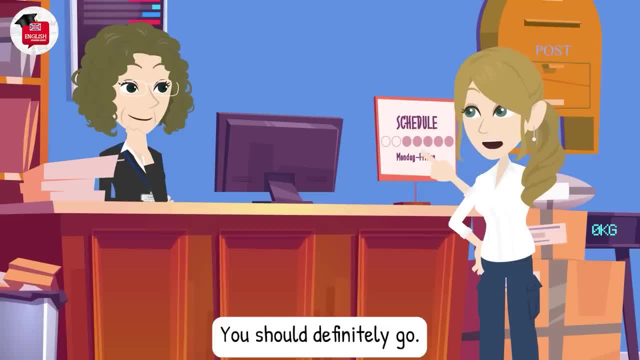 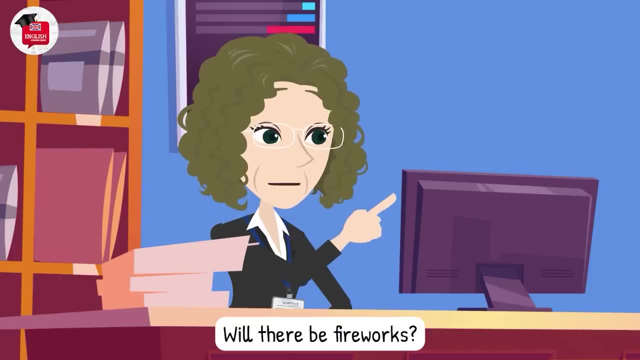 I'd also want to visit Chinatown. You should definitely go On Saturday. there will be a Lunar New Year parade. On Saturday, there will be a Lunar New Year parade. Mark and I are leaving. Will there be fireworks? Yes, Do you want to go with us? 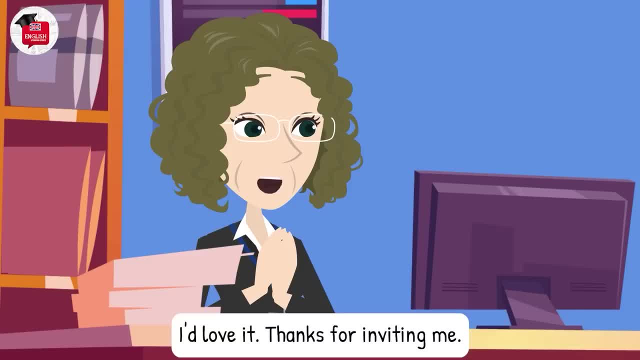 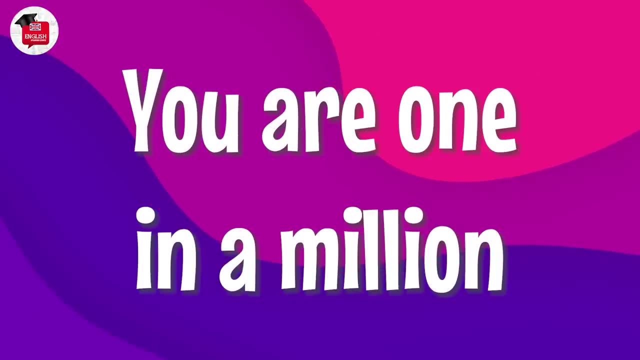 Yes, Do you want to go with us? I'd love it. Thanks for inviting me. I'd love it. Thanks for inviting me. I'd love it. Thanks for inviting me. You are One in a Million. You are One in a Million. 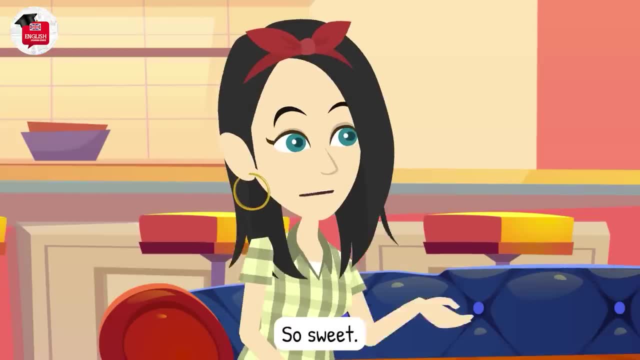 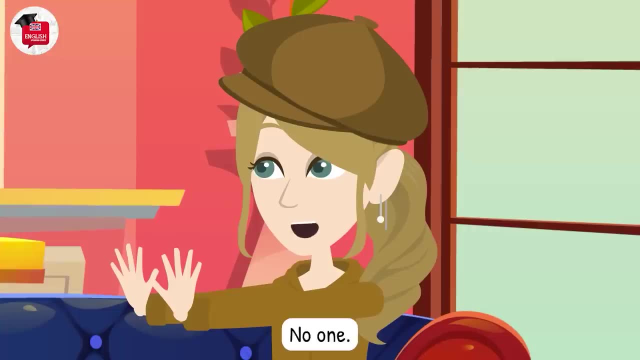 This card says you are One in a Million, So sweet. Is it okay if I give this to Jim? Is it okay if I give this to Jim? Who is Jim? No one, Don't try to trick me. Surely Jim must be someone. 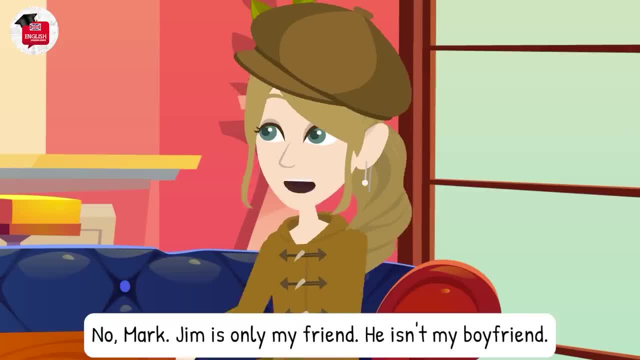 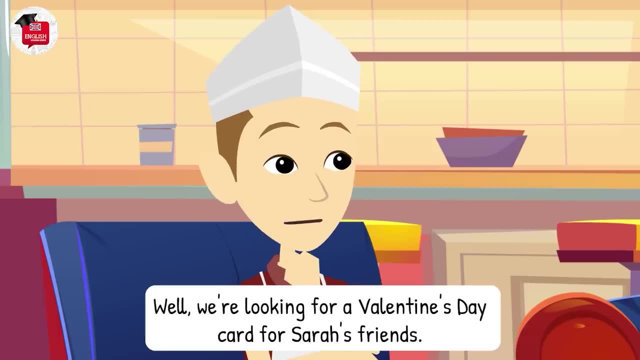 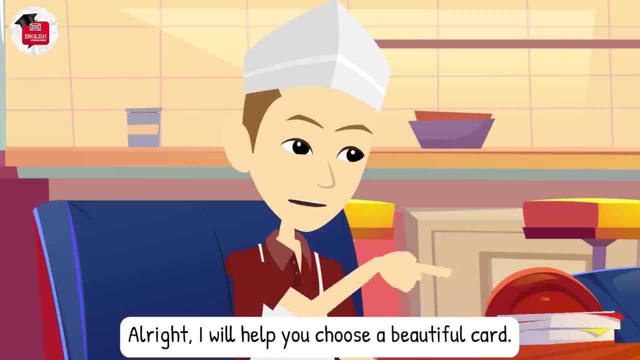 Maybe he's even someone special, right, Sarah? No, Mark, Jim is only my friend. He isn't my boyfriend. Well, we're looking for a Valentine's Day card for Sarah's friend, Mark. don't tease me, Alright, I will help you choose a beautiful card. 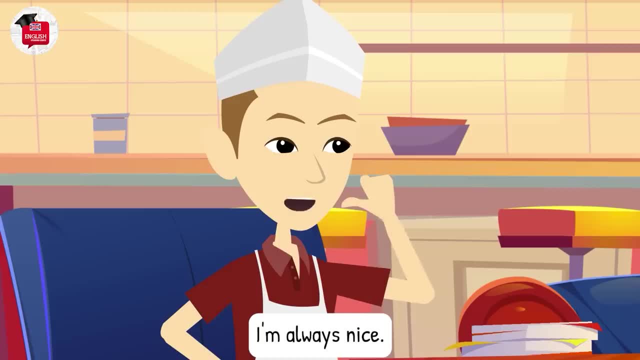 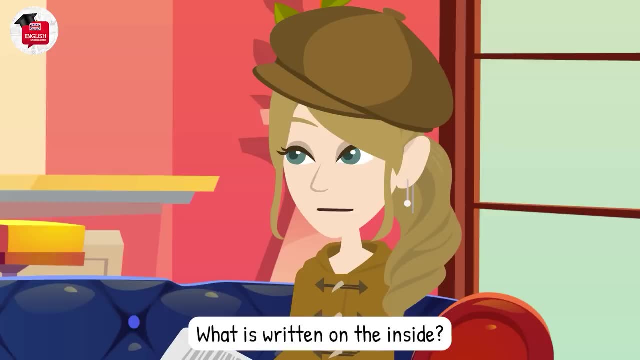 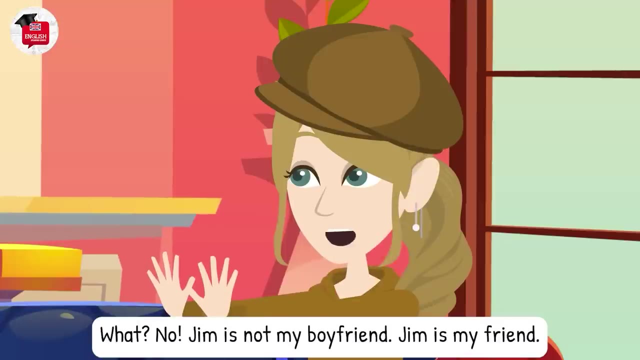 Okay, but be nice. I'm always nice. This one is adorable. Let's stay buddies till the end. That's adorable. What is written on the inside? I love you. That's great What? No, Jim is not my boyfriend. 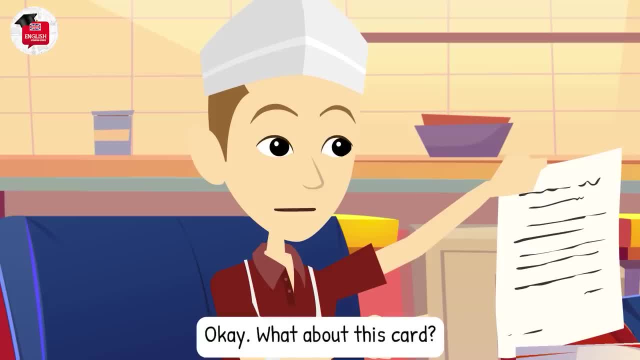 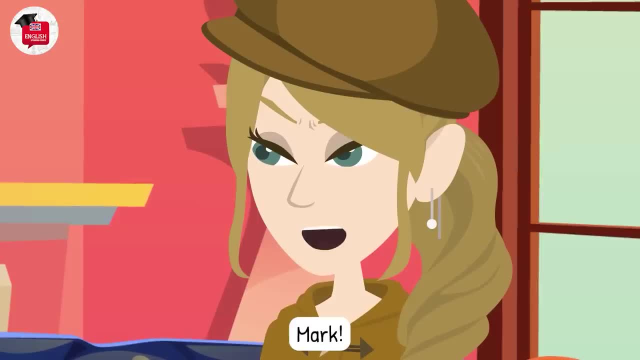 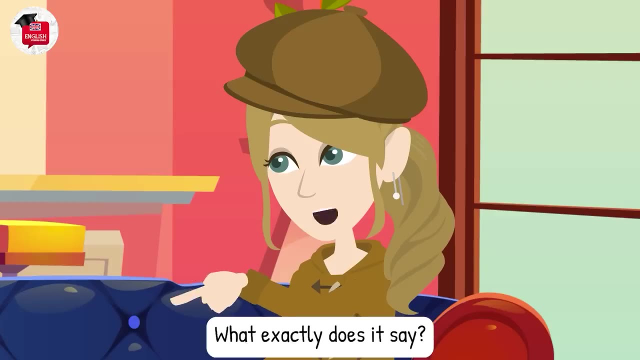 Jim is my friend. Okay, what about this card? What does it say on the inside? The card says: Hello, sweetheart Mark. Alright, alright, I found one. It has a sweet message. What exactly does it say? Does it say: I have a crush on you? 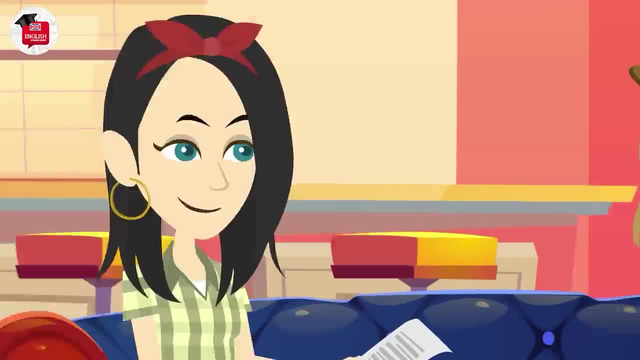 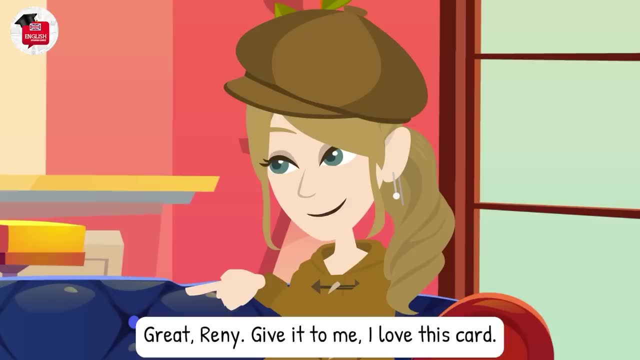 It says thank you for being my friend. Is that all? That is all. This card is not romantic at all. Great Rennie, Give it to me. I love this card. Yeah, you can write my own special message. 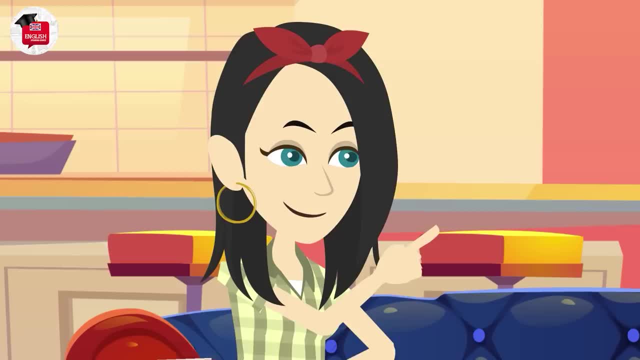 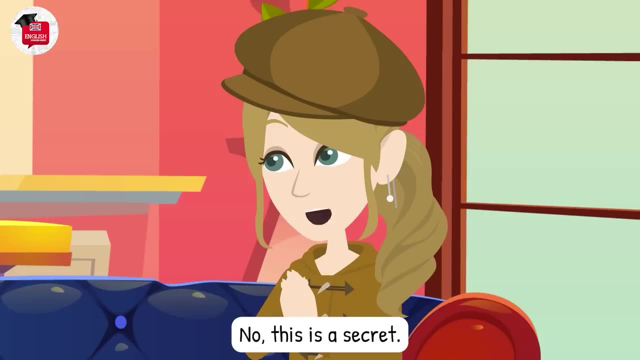 Your friend Sarah. Okay, I'm done. Bye. Good, Jim will treasure your card. Read it to us, Sarah. No, this is a secret. Hey, I'm your brother. You're also a good brother, Thanks. 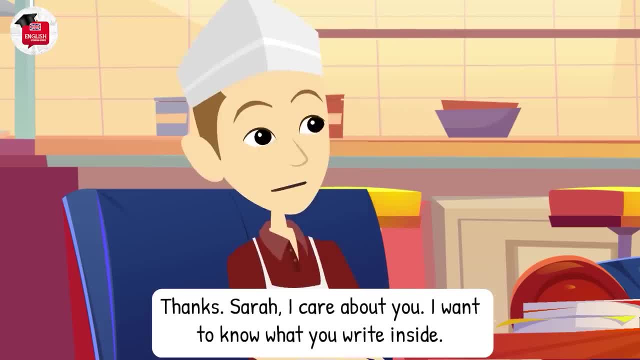 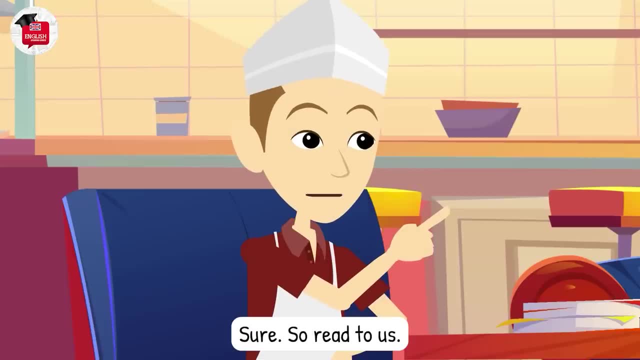 Sarah, I care about you. I want to know what you write inside. Thank you very much, Mark. You are a great brother, Sure, so read to us. You know, Mark, you always make me happy Because I am your brother. 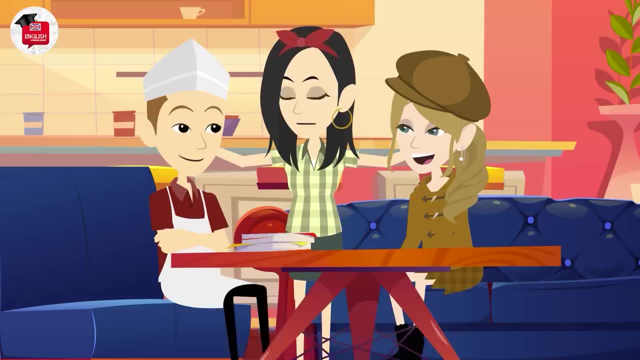 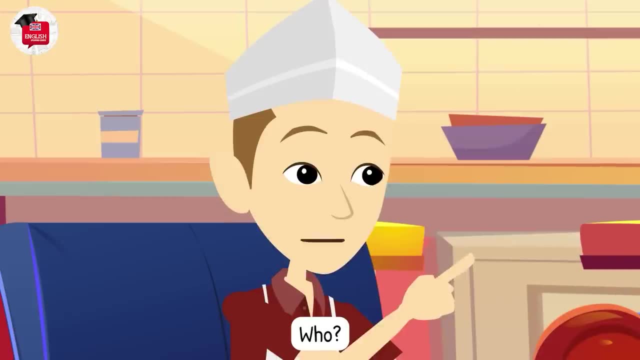 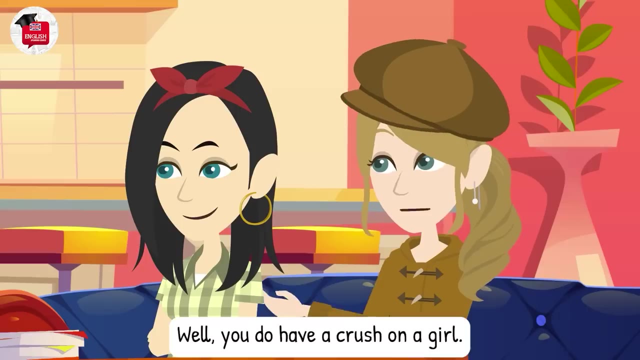 You two are so sweet to each other, Let me give you a hug. Thank you, Uh-uh, Mark, you can also offer someone a hug Who? Someone special to you? No one is special. Well, you do have a crush on a girl. 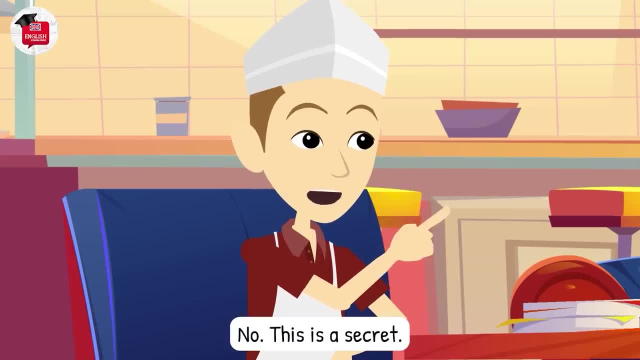 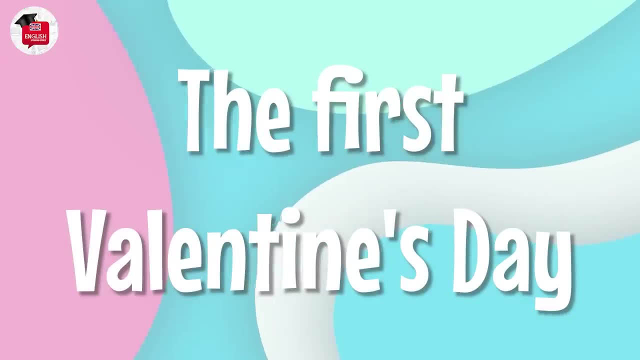 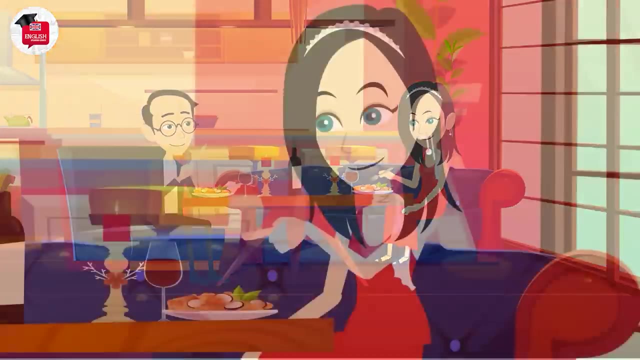 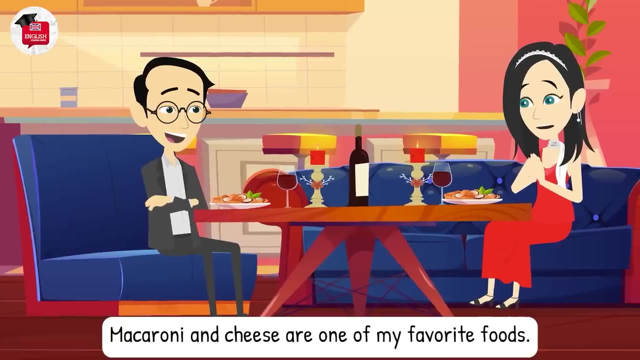 Really Tell us about her. No, this is a secret. The first Valentine's Day- Wow, this dish is so delicious. Yeah, I'm glad you like it. Macaroni and cheese are one of my favorite foods. I can't believe you cooked this dinner. 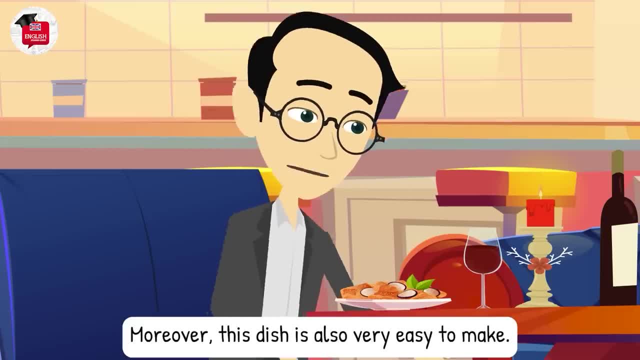 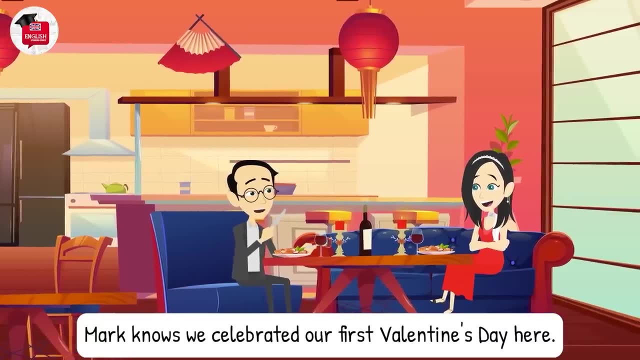 Moreover, this dish is also very easy to make And, Mark, he can do it all by himself, even like you, use his kitchen. Mark knows we celebrated our b-day. We celebrated our first Valentine's Day here. For us, this restaurant is a special place. 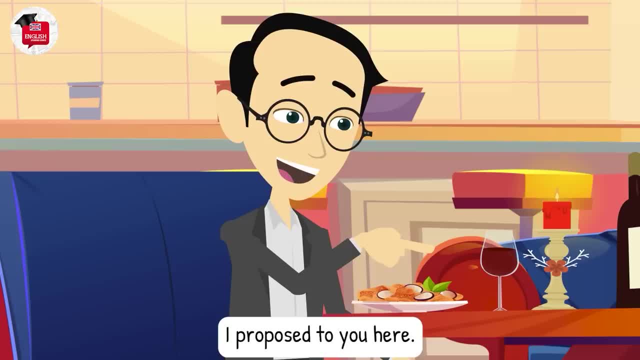 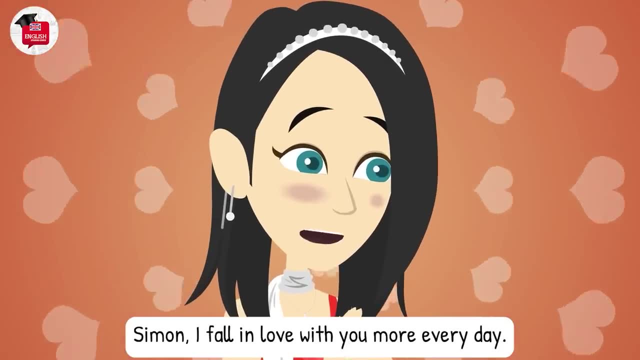 Yeah right, We had great memories here. I proposed to you here. It was the happiest day of my life. Aw, Simon, I fall in love with you more every day. I love you too. Do you remember the first Valentine's Day we spent together? 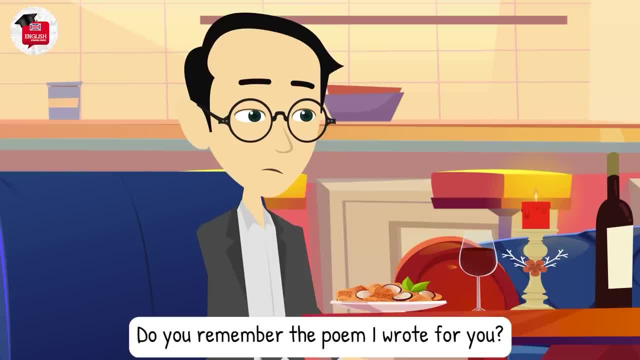 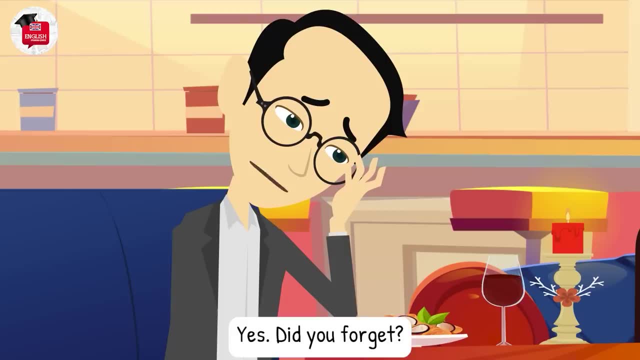 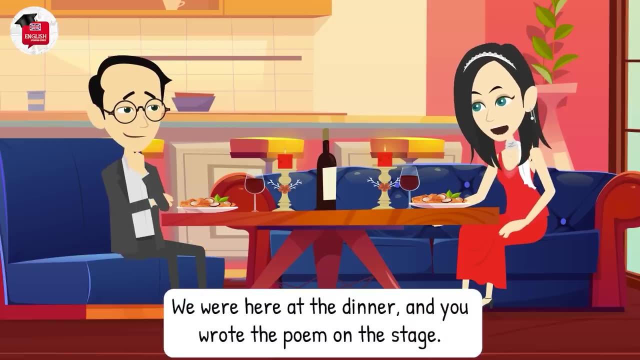 Obviously, I never forget that day. Do you remember the poem I wrote for you? Did you write a poem for me? Yes, Did you forget? No, honey, I was just kidding. We were here at the dinner and you wrote the poem on the stage. 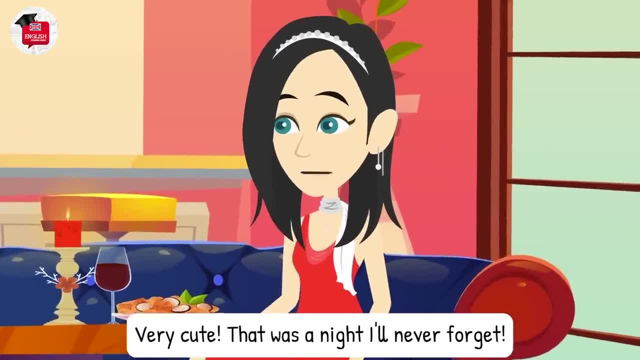 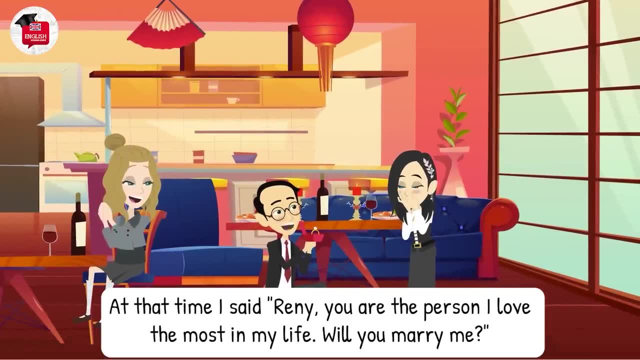 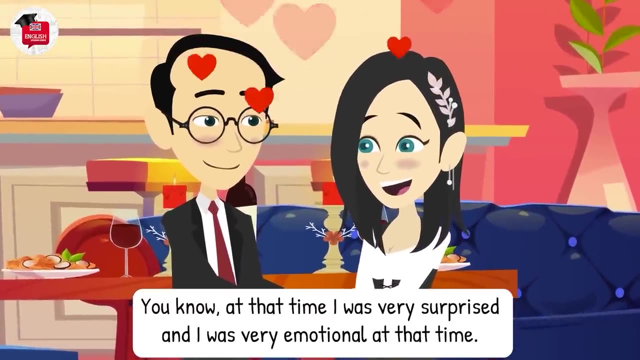 I was tense at that time. Very cute, That was a night I'll never forget. At that time I said: Rennie, you are the person I love the most in my life. Will you marry me? You know, at that time I was very surprised and I was very emotional at that time. 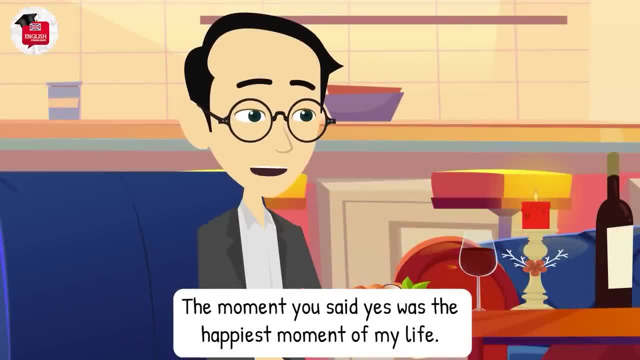 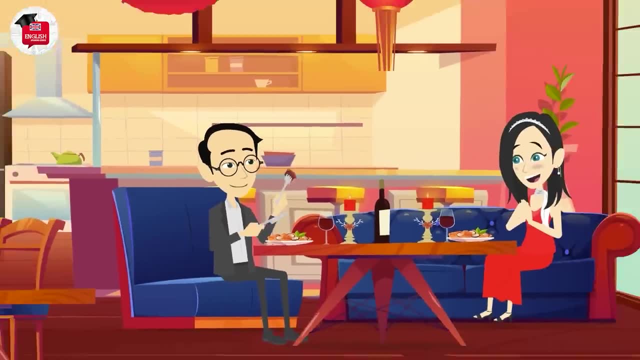 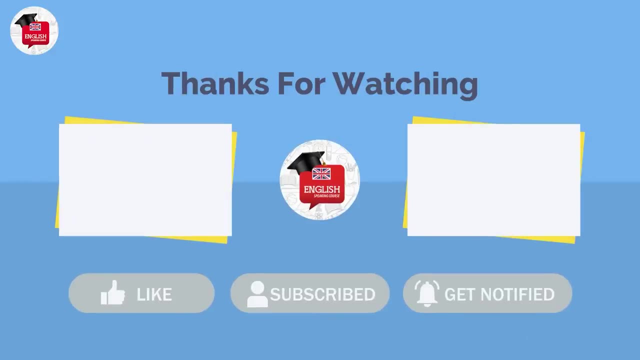 The moment you said yes was the happiest moment of my life. I was so happy that you would be my husband. Thank you for watching. Please give us a like, share and comment. Click here for a more useful video. See you in the next video. 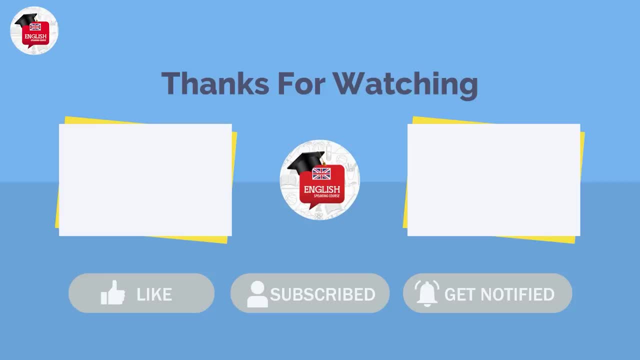 Thank you for watching. See you in the next video.